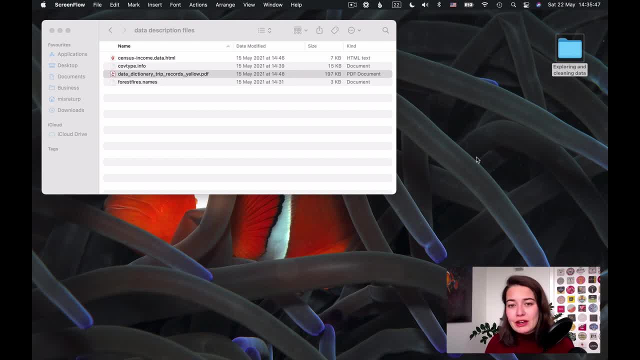 I can come up with when it is time for future engineering and if I, you know, need to create some new features. So just to have the, just like a small advice for me. you know, if you have any questions, just let me know in the comments below, And if you have any, 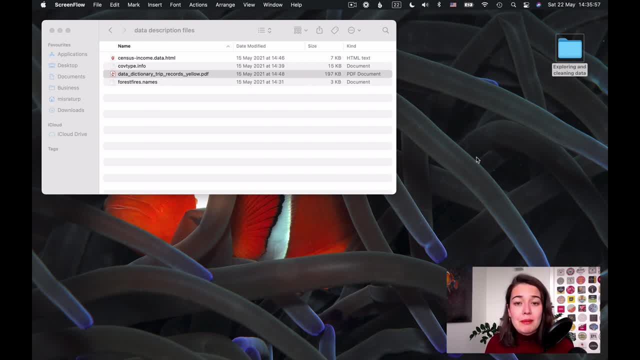 questions, just let me know in the comments below. And if you have any questions, just let me know in the comments below. And if you have any questions, just let me know in the comments below. Keep these two questions in your mind, like how am I going to clean it and how am I going to create new features? 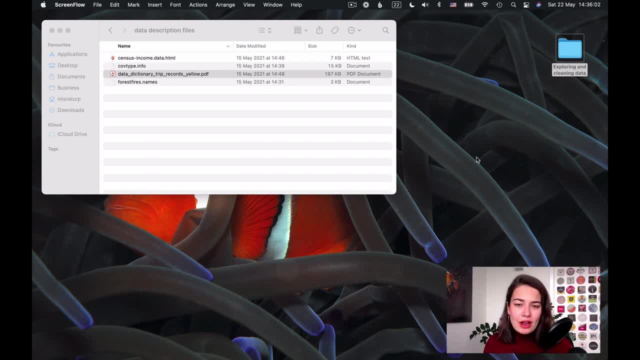 in the back of your mind while you're doing the exploration Don't have to be very formal, it's just some things that you need to be thinking about in the background. So, but let's start with the technical part. So the first and foremost- again I feel like this- is: 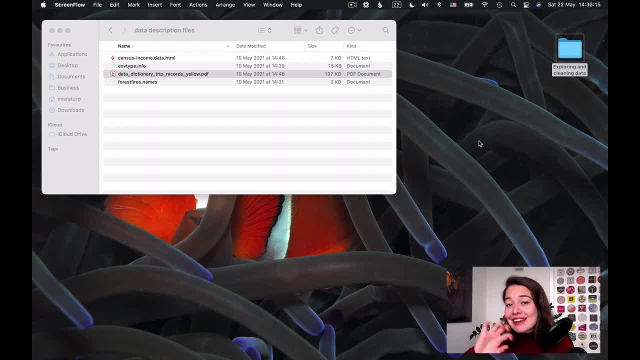 the second, first and foremost thing that I said. but in the technical side of things, the first thing that you need to understand is when you find a dataset in the wild and out in the open on the internet, you really can't understand a dataset by itself. Of course, it could be a very 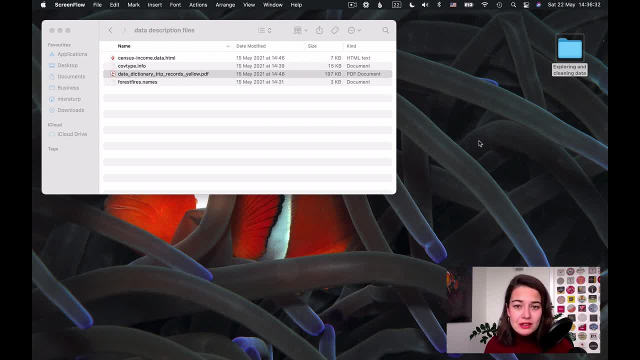 simple dataset, a toy dataset, like a small one, very easy to understand. But most of the time you're going to be seeing data that has some column names that you don't understand. that is kind of, or it has values that you don't understand. It could have a different unit. 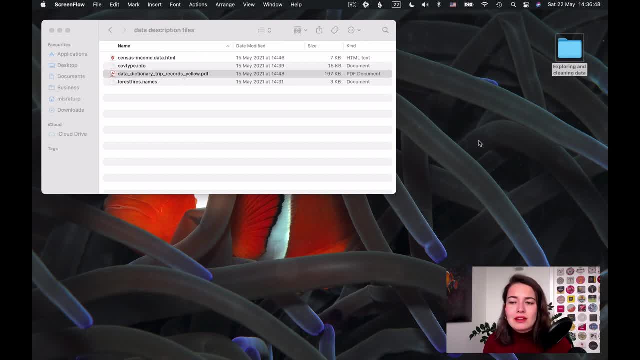 the column values might have a different unit. you know the way the things are represented could be different, So likely there will be things that you don't understand. but you can. you will not fully understand, especially if it's in a new domain, that you never wrote them before. 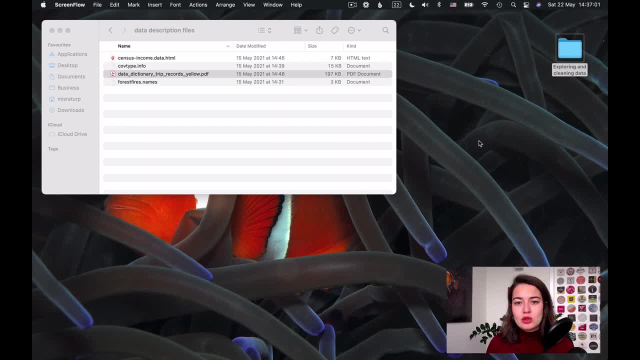 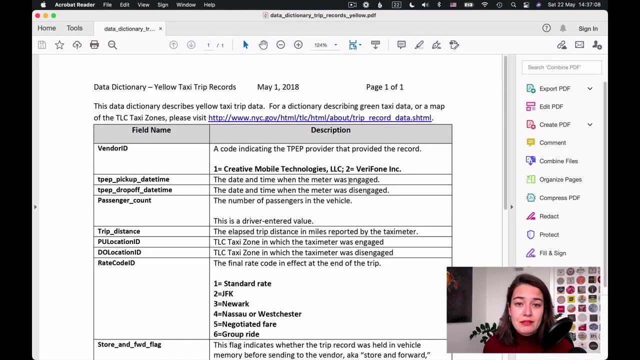 So how we solve this is: there is always going to be some explanation files for the dataset that you're finding. Just want to show you some examples. like you know, it might look like a PDF like this one And it basically tells me for this specific dataset that I found online. 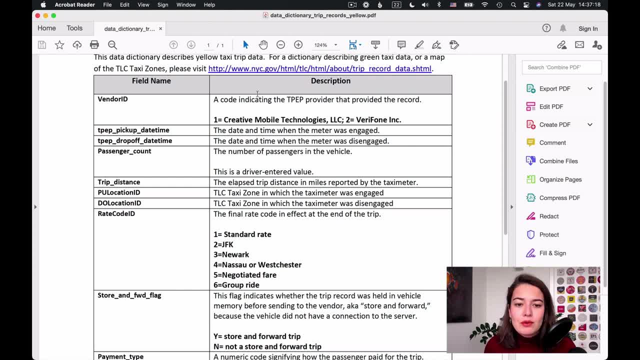 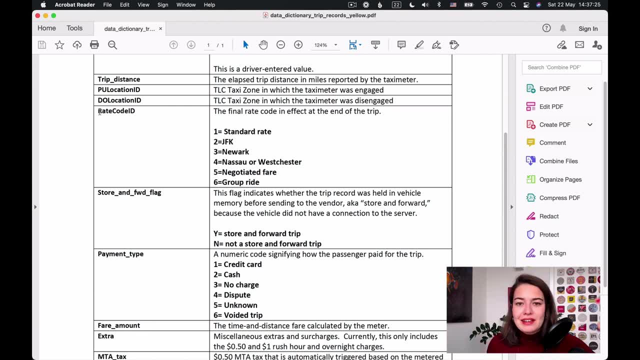 each field or column name and what they mean, what the do the different values for this column mean? for example, it says it has a rate code ID. I mean this is a data set I used for my course hands on data science. 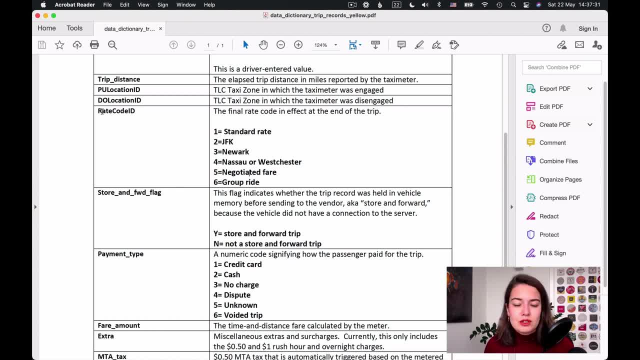 It's a New York City taxi data set. So it's basically like all the trips that happened in the in New York in like a whole month or something like that. So apparently this rate code, you know, and if it means if it's one, it means the standard rate, if it's two, I guess it means that they're. 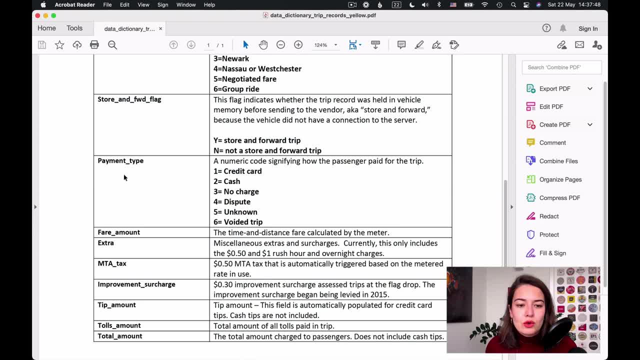 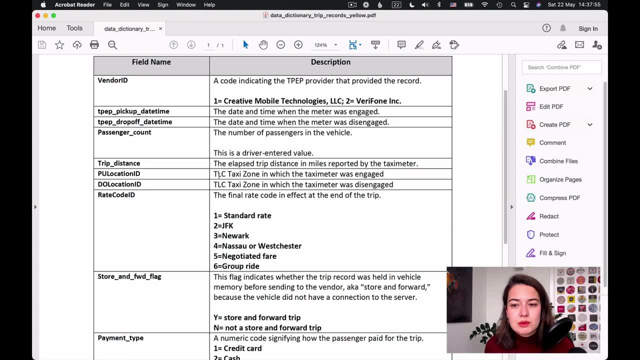 going to JFK or New York or you know similar things, or the payment type you know. if you just are looking at the data, you will not be able to understand this, So it's important to see these explanation files. you're always going to find them somewhere. So, as I 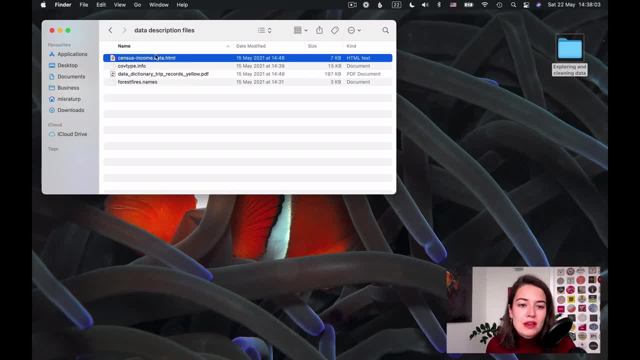 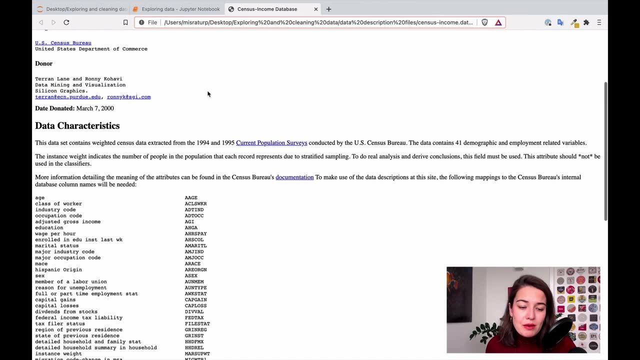 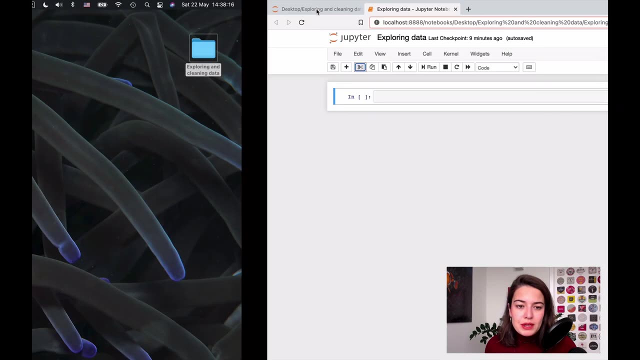 said it could be in a PDF format. it could be apparently HDMI for HTML format. So it'll just generate a website for you or a web page For you can see. you know what does this mean, What does that mean, etc. get some indication of like what things mean. Or it could also be just like random. 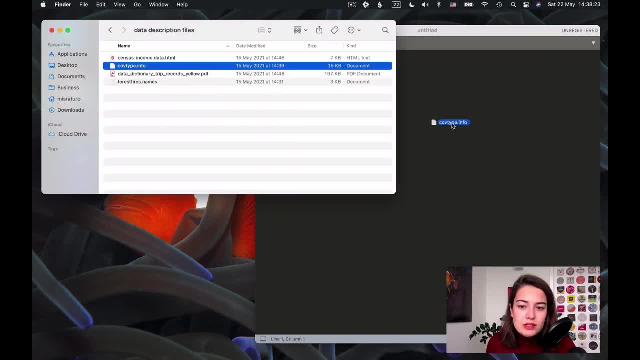 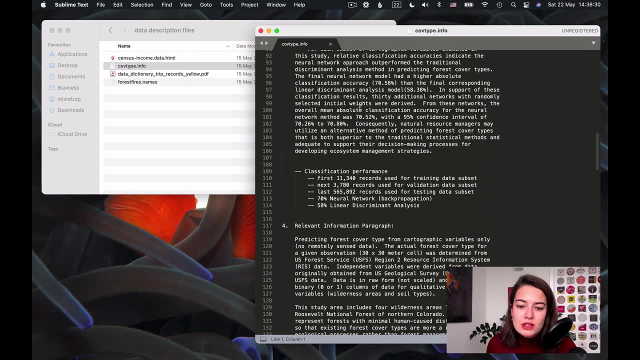 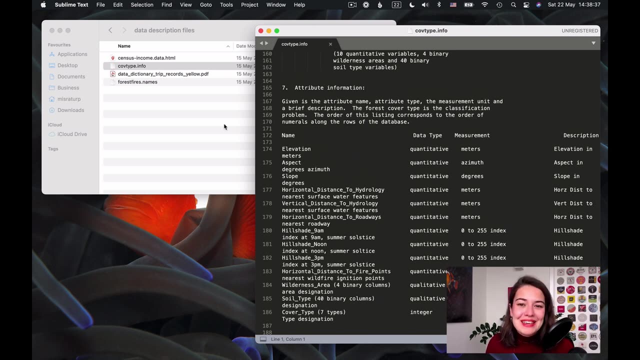 text files, So we can see this one, For example- so this is just an explanation- title of the database sources. how can you use these, etc. etc. And then here the attributes. So, as I'm saying, you know the columns can be in a lot of. 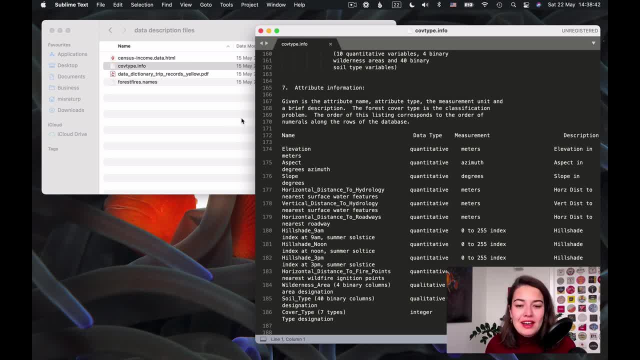 things. So it could be columns, fields, attributes, features. Yeah, we just need to kind of find this like table that explains what each column is. Sometimes they give you the data type, Sometimes they give you the the range of the columns. 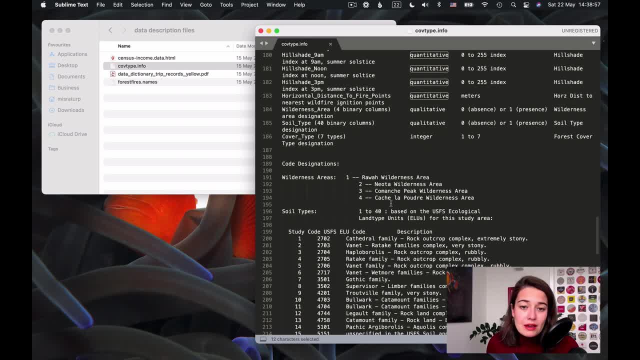 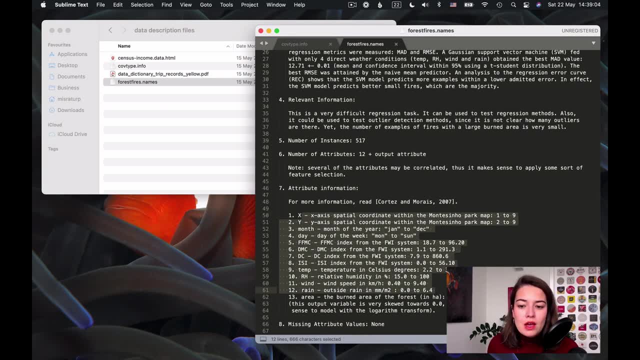 Yeah, that's also possible. Yeah, this one is like that. Or, you know, this one is a different one that also has information about the columns. So this is the first thing that you need to find If you are working in a company or if you're getting the data set from a different team. so you didn't. 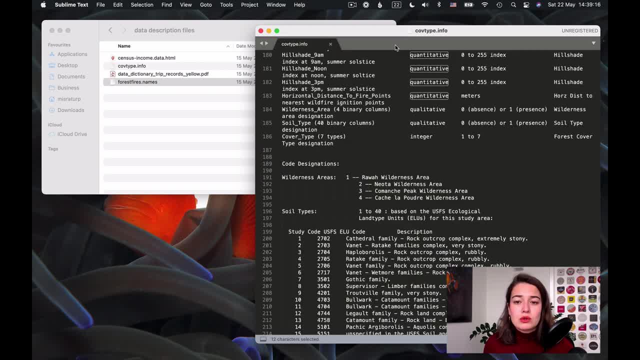 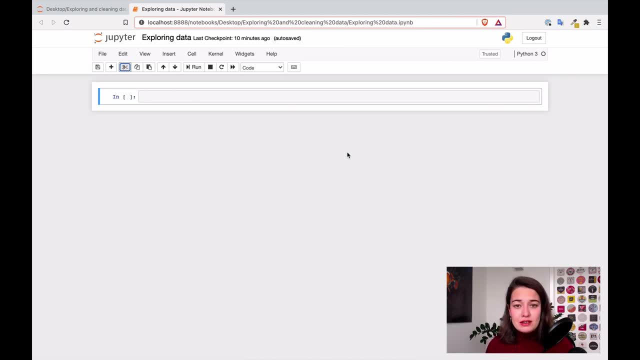 find it online. let's say in that case you first want to understand the data set, like kind of open it on a Jupyter notebook like this, read it and try to understand what's going on in the data set And try to understand as much as you can And write down questions about what you don't understand And then go and find. 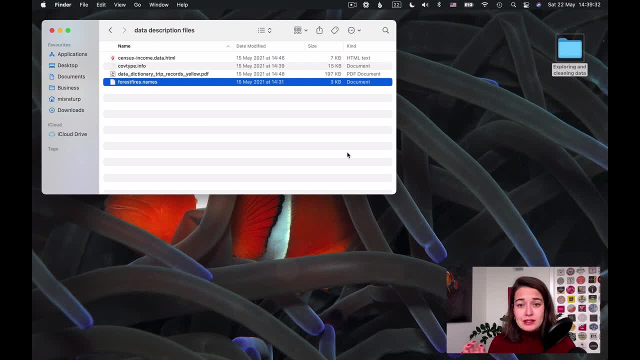 the people who are responsible for this data set and ask your questions, Like this happened to me before, And what I did is basically like just reach out to the person who sent me the data file And she was like Yeah, I'm sure, but someone else. 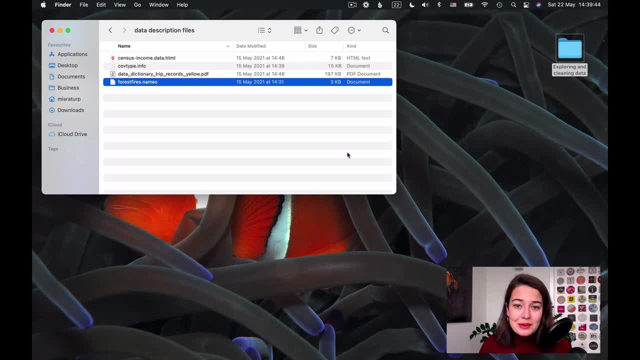 sends me these files. I don't really know much about them. So I was like, Okay, can you give me the name of the person who sends you this files? And I talk to that person is like, Yeah, but I just downloaded from a system, So I don't really know. 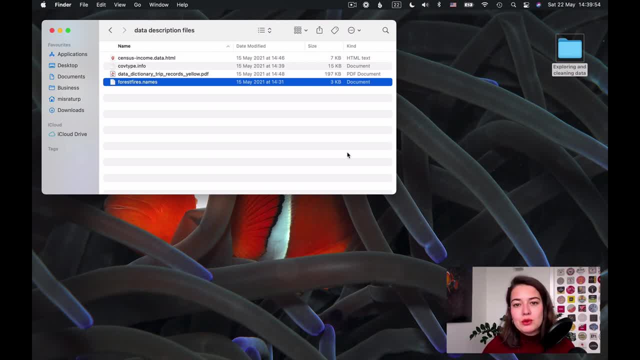 how it's collected. So then I'm like, okay, I'm like okay, I'll just go to the people who created the system that collects the data. Let's say it's the engineering team. So then I go and talk to the engineering team's head. 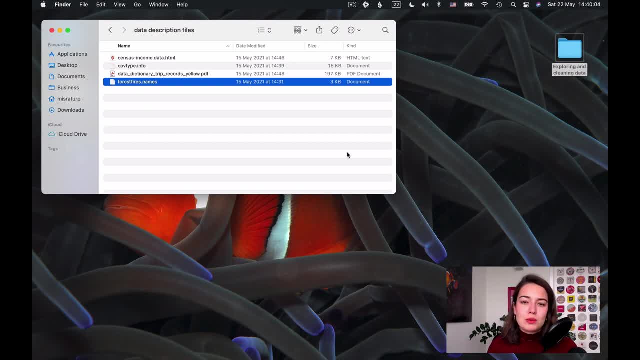 and he points me to the person who set up the system or who's responsible for the system that collects the data. And then, you know, I ask him my question. So sometimes it takes a little bit of time to get the data, to understand the data, et cetera. 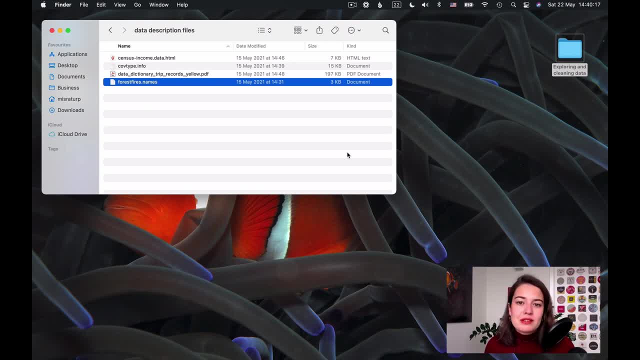 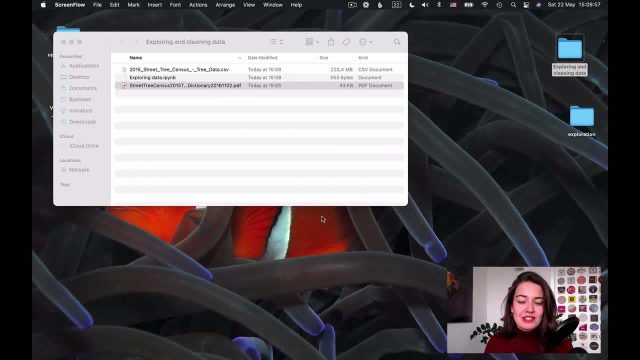 and kind of feel comfortable with it. But this is very important because otherwise you know, you don't know what you're working with. The data set that we're going to work with today is called the Street Tree Census data set. So I don't know if you're familiar with what a census is. 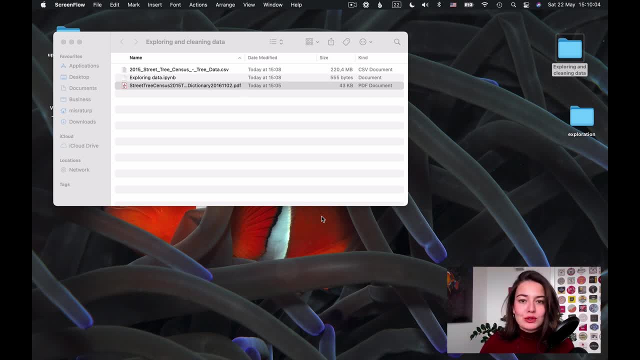 It's basically when they go. well, what they used to do is go from door to door, ask people how many people live in your household, how many of them are adults, how many of them are children, how many of them are working. 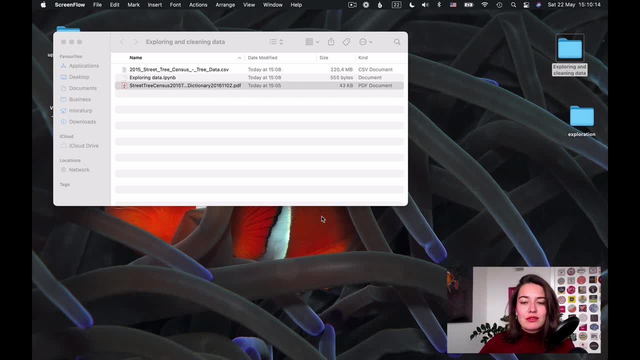 how much money are you making? So basically, kind of like getting a lay of the land of like who lives in a certain city or a country. But they did that for trees in New York, So I might've mentioned this before, but there is a New York City. 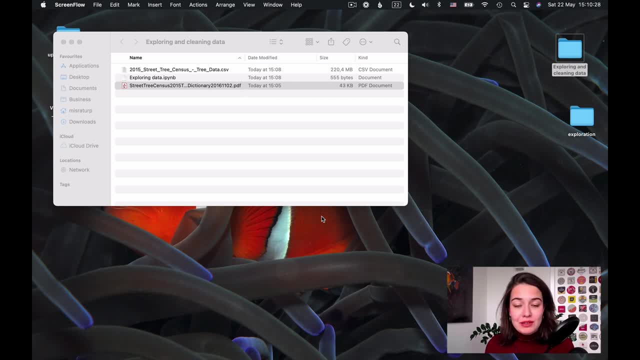 open data platform where you can download a lot of different types of data sets, And this is also where I found this. I think it's really amazing. It's a really cute data set, So let me first start with reading it on my notebook. 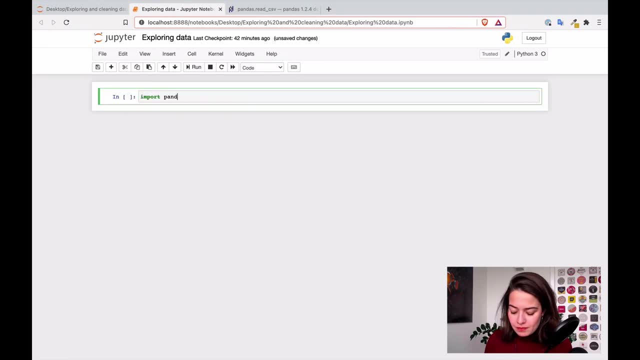 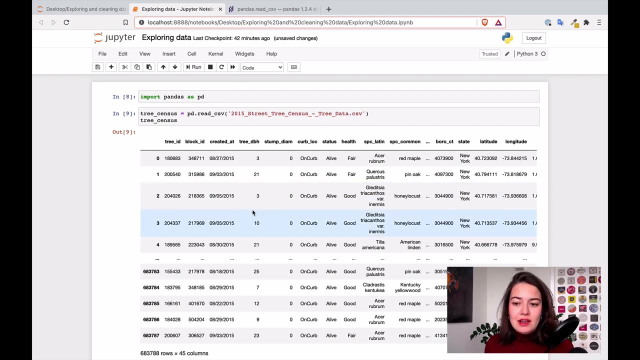 and then we start looking into it. All right, so this is a data set. It has a lot of columns. As you can see, there are the three dots. It means that it hasn't even been able to show me all the columns, but there is actually a solution to that. 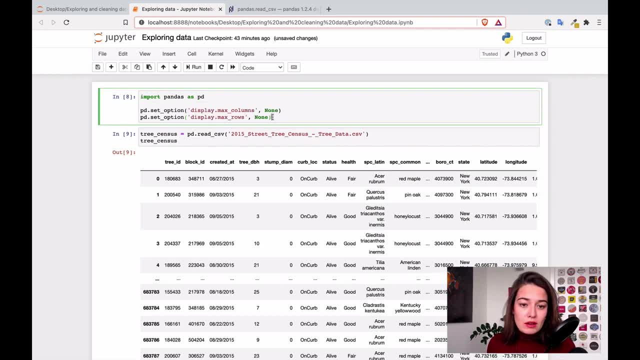 If you change the settings to you know how many columns that you want to show. I mean this basically says for Panda, set the option to maximum columns, that will be shown to none, So then it will display all the columns. I don't want to set the option to show all the rows. 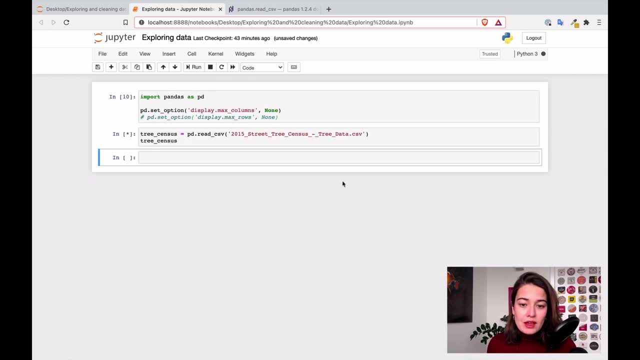 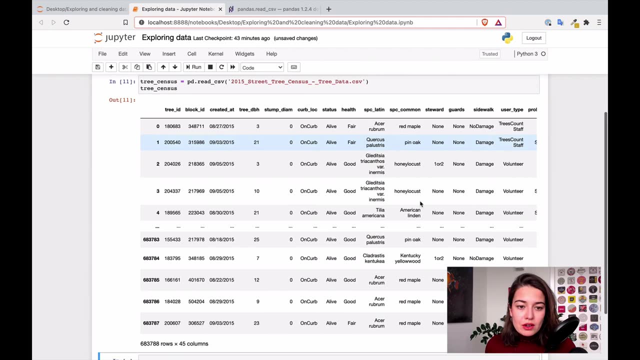 because that might be a little bit too much. So I'll change the setting and then have it: show me all the columns. And yeah, I can see all the columns now. So, as you can see, I have a lot of columns And some of them are not really obvious what they are. 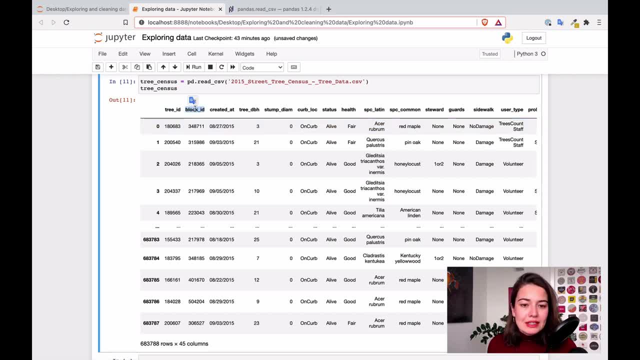 So, for example, this tree ID- okay, pretty easy Block ID, yeah, you know, I kind of understand what it means- Created at tree DBH, for example. I don't know what that is. So, to understand what these things are, as I said, 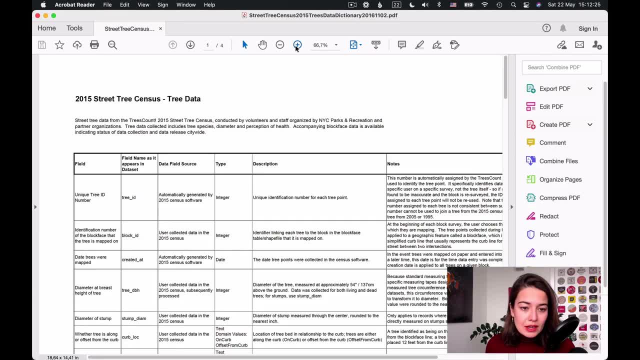 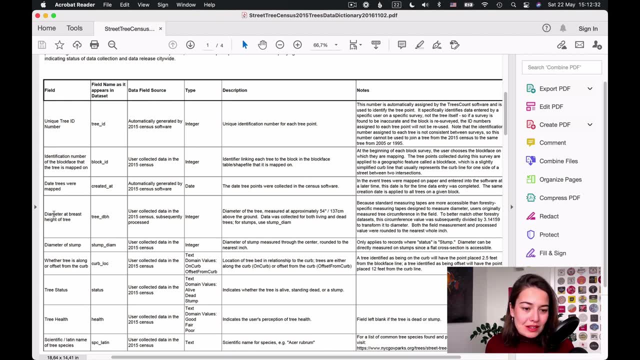 we have the file with us here, Very tiny font size, but at least we can understand what things are. So, for example, 3DBH apparently is a diameter at breast size. So I guess the breast height of a person, Diameter of the tree measured approximately. 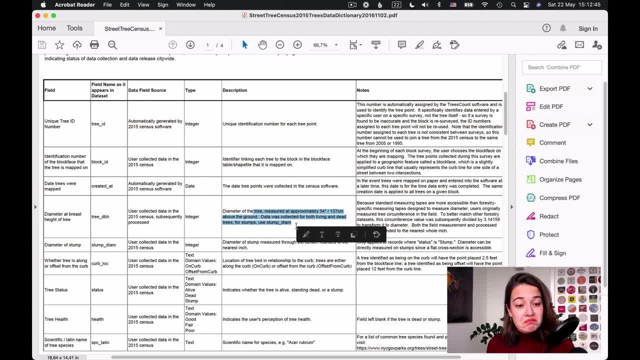 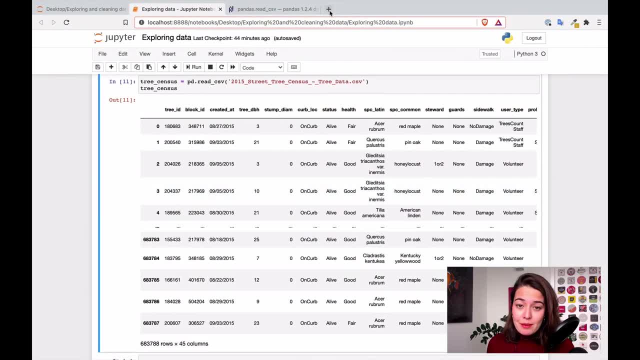 137 centimeters above the ground. Okay, that's cool Diameter of the stump. I don't really know what a stump is, So when stuff like that happens, what you need to do is Google tree stump- See what it is. Tree stump tree has been cut felt. Okay. Okay, that's good to know. Yeah, Whether the tree is along or offset from the curb, Tree status indicates whether the tree is alive, standing dead or a stump Tree health. 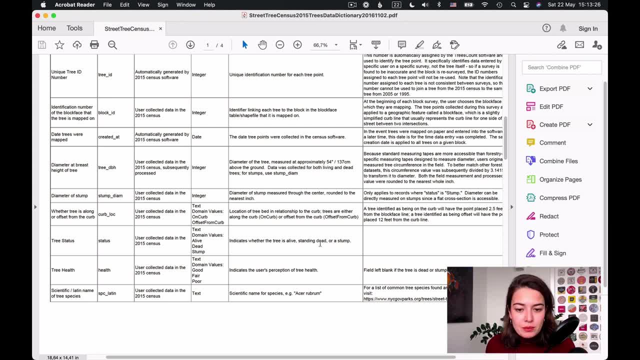 Oh, okay, So the tree might be a stump or not a stump. So if a tree is a stump, I'm guessing- then we only get the diameter of the stump. Otherwise we do not. We do not have that. So this is an assumption that we're making. 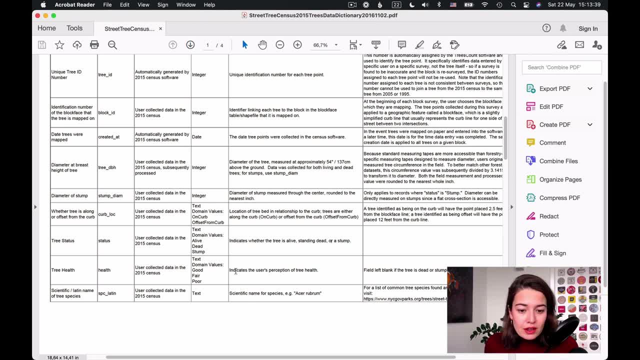 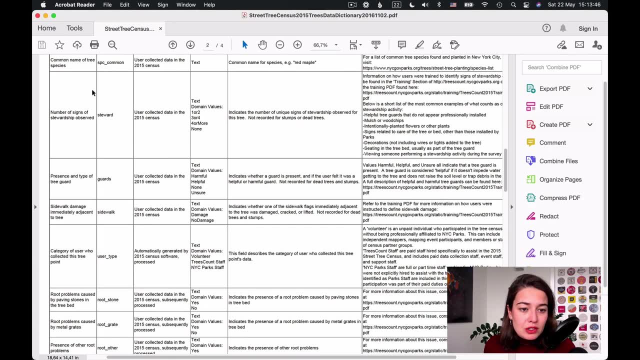 but we'll see if that is the case or not. Tree health indicates the user's perception of tree health. Scientific name: Common name of tree species. Number of signs of stewardship observed. And that is indicates the number of unique signs of stewardship observed for the tree. 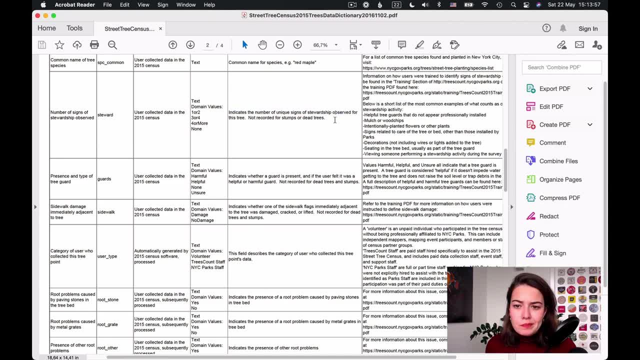 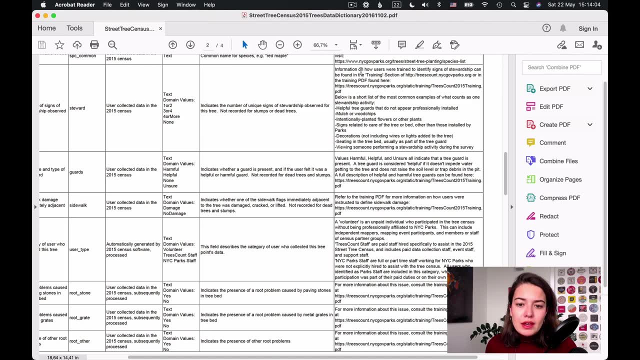 not recorded for stumps or dead trees. Okay, So I guess stewards are people who are taking care of the tree. That's what I understand. Good Presence and type of tree guard. Sidewalk damage immediately adjacent to the tree. 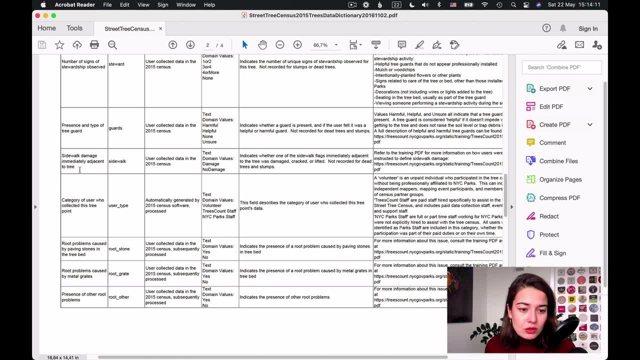 Category of users who collected this tree point. All right, So this is good information. Now we know more or less what these things are, So let's look into our data set a little bit in more detail. So at first it might seem a little bit overwhelming to know where to start. 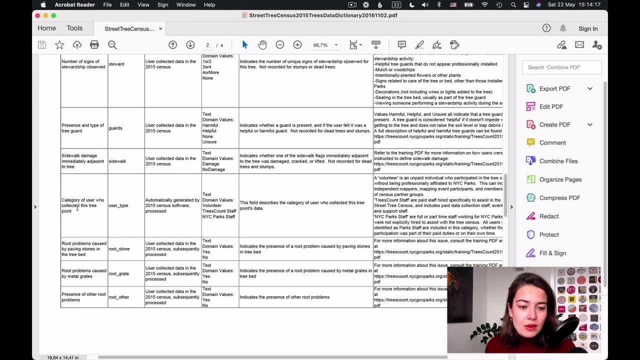 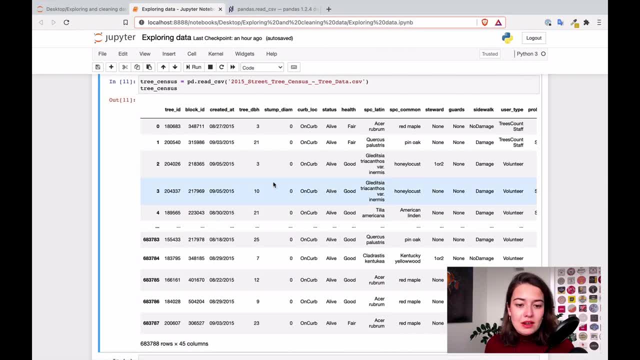 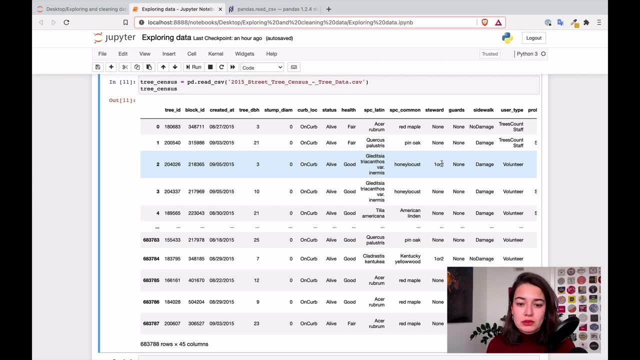 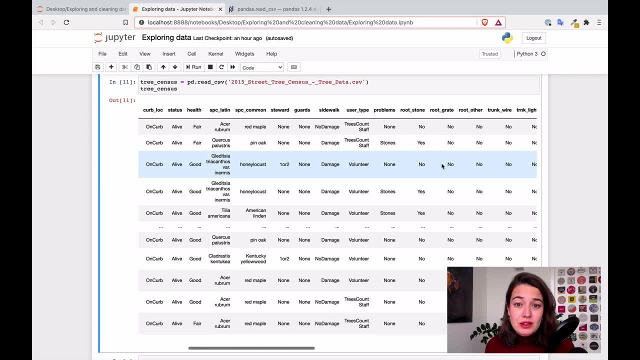 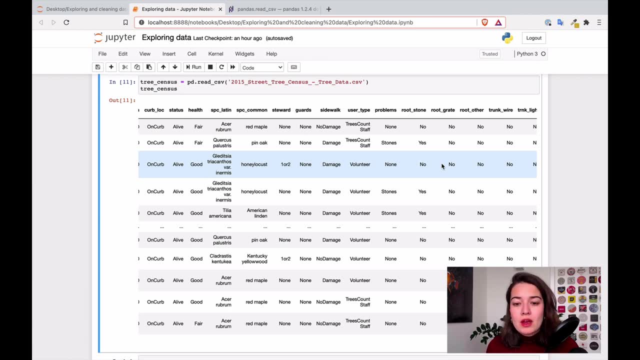 we have a lot of column names And you're like, wow, this is going to take a while to explore this data set, to understand what's going on. But I think one important thing is to understand what your priorities are. So let's say generally, I just want to understand the situation in New York about trees. how 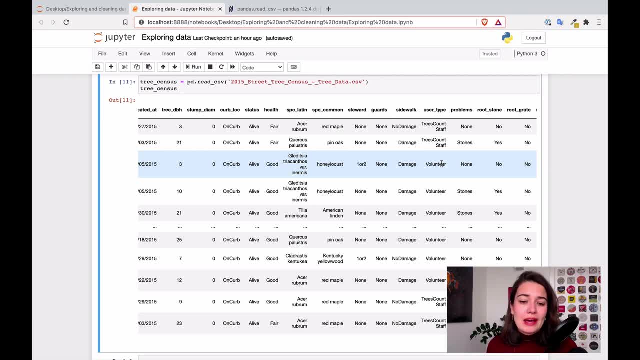 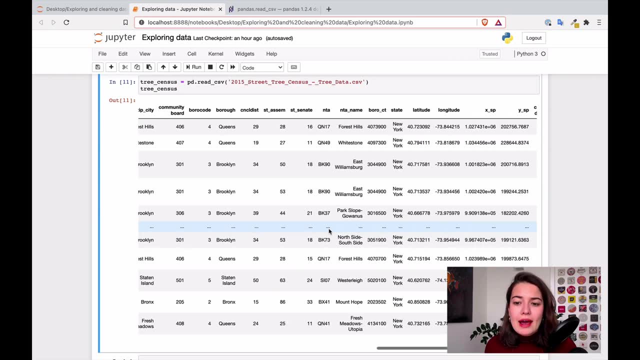 much of them are healthy? how much of them are not? I just want to get a general feel of the trees in New York, So I'm going to start with a tree. Let's say that I was going to start out in the west side of the state, or New York City. 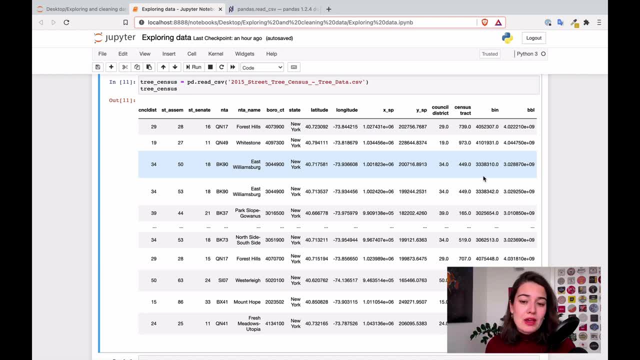 sorry, So then I wouldn't really be caring about their location. So when that happens, you know, then you can basically just get rid of all the columns that are giving you some information of, like, which state they're, in which borough they're. 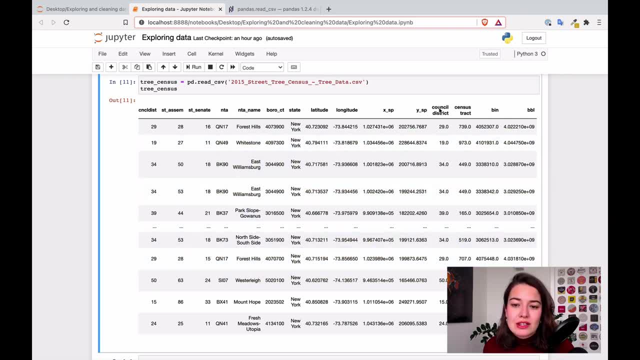 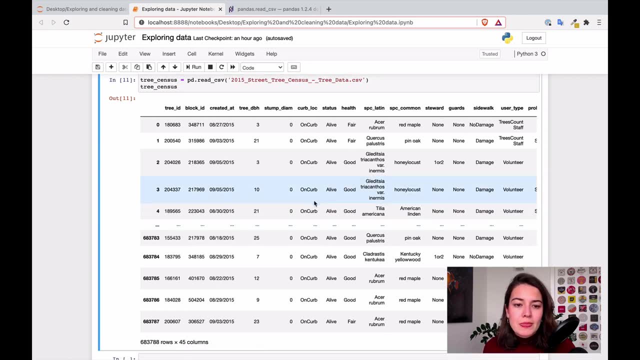 in which city, which street they're in, et cetera, Longitude and latitude of the tree, et cetera, Et cetera. So for now I can actually get rid of these things And I will make a list of all the columns that I'm interested in. 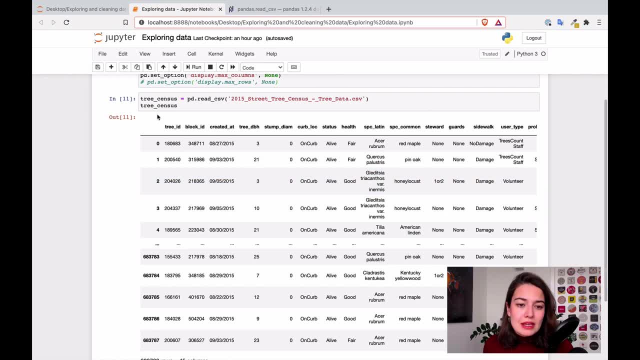 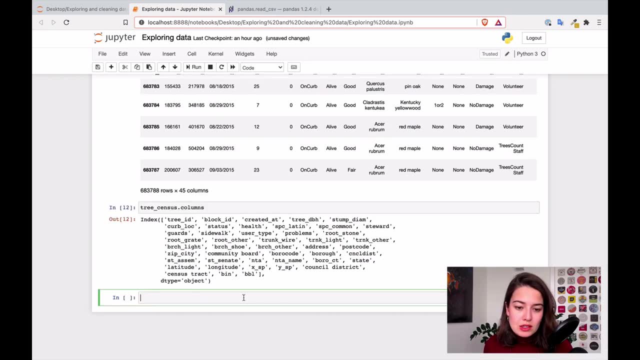 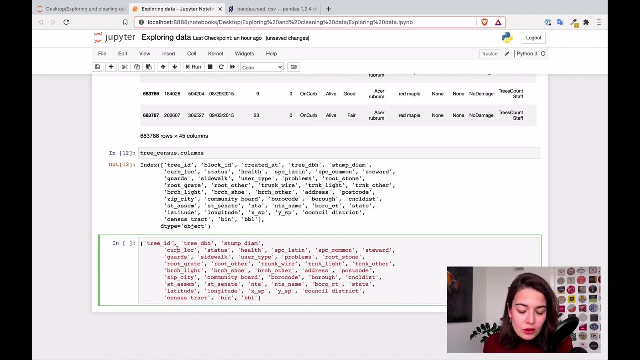 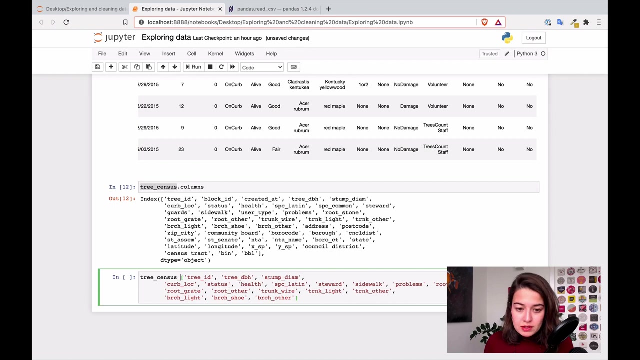 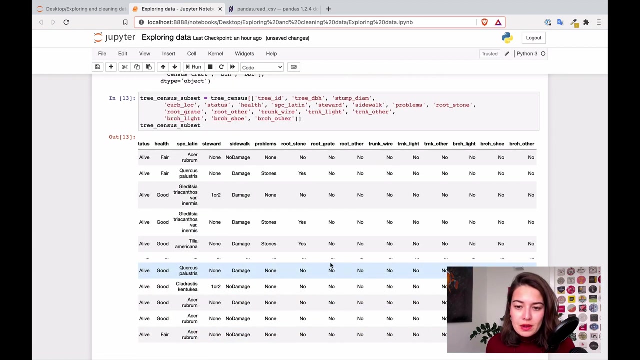 � jumped off screen yet, studioёр色 And to make it easy, what I use is the columns function, it will give me all the columns so it's easier for me to delete the ones that I'm not interested in. So this is more manageable, these are all basically if there is a problem caused by 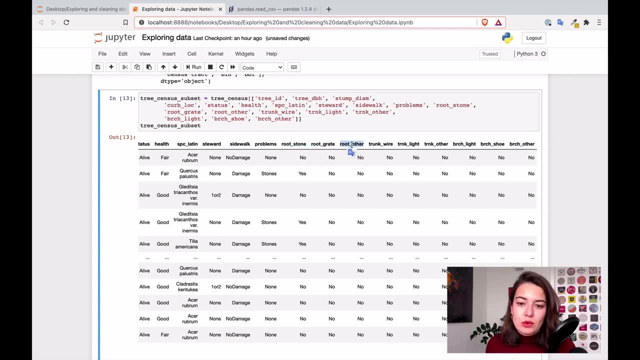 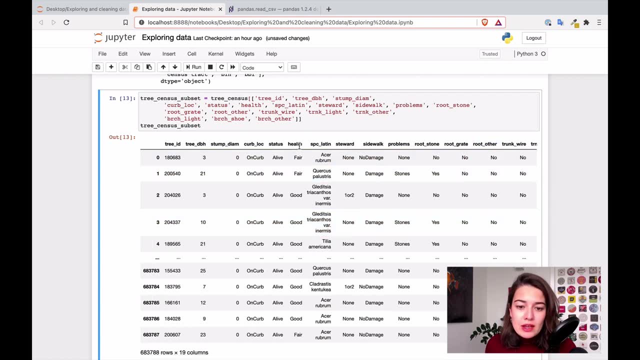 a stone on the root. if there is a problem on the root caused by a grate or other, same with the trunk and same with branches. That's easy to understand The Latin name of the trunk, The tree, If the person who was collecting the data thought it was healthy or not. 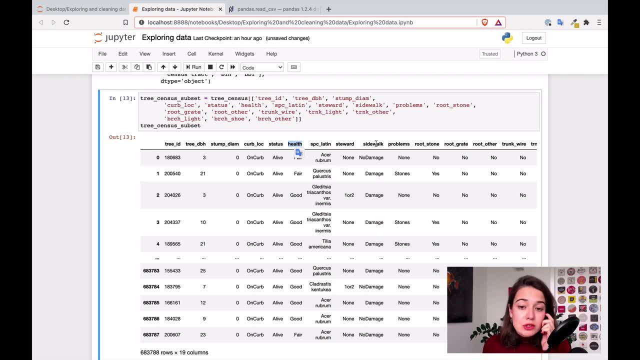 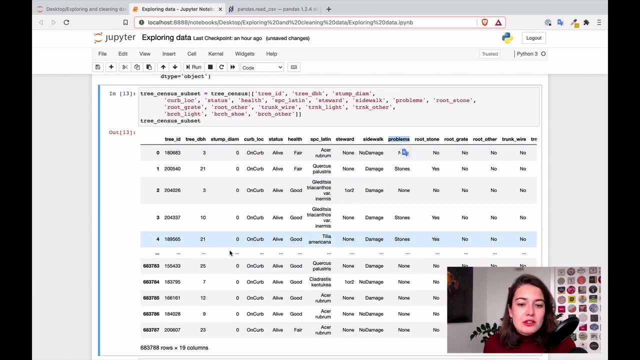 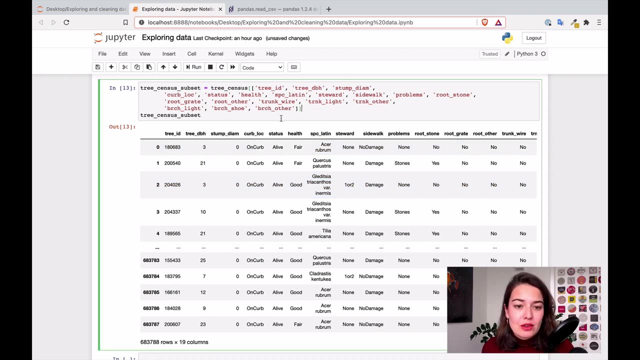 The status of the tree If there is damage on the sidewalk right next to the tree. If there are any other problems, Okay, This is good, I can work with this. So one of the first things that I want to look at is the numerical values. 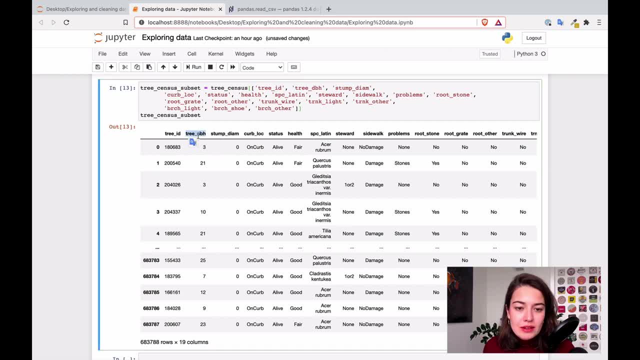 So the numerical values that we only have are the diameter of the tree and diameter of the stump. But, as I figured out, if this tree is a stump, so if it's cut already, then we do not have the diameter for it, Which makes sense. 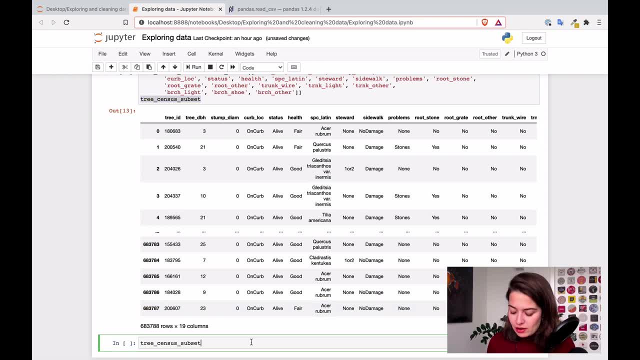 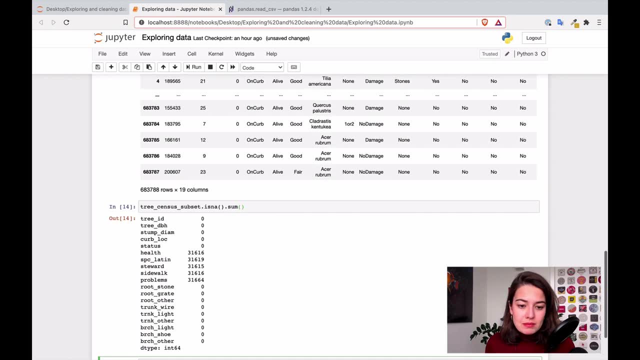 But actually, even before that, I want to see if there are any null values. This is how I can see if there are any missing values or not. So it looks like with health we have a bunch of missing values. So how many values do we have? 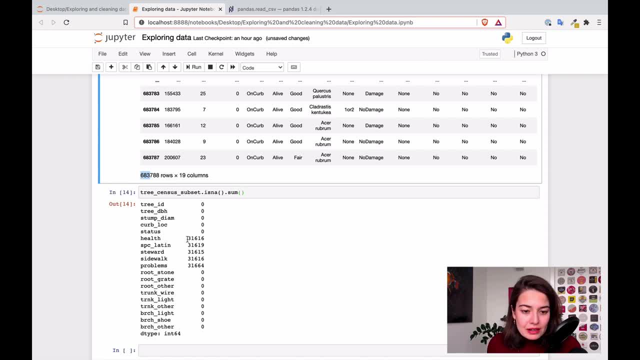 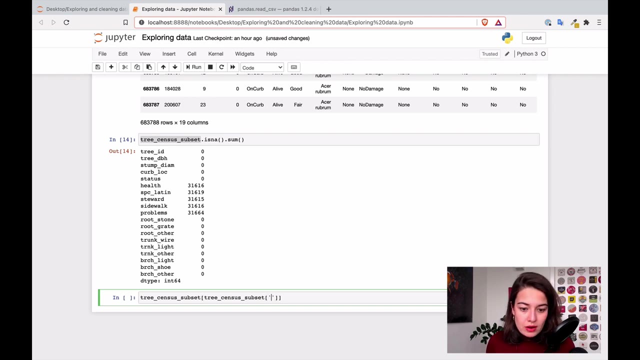 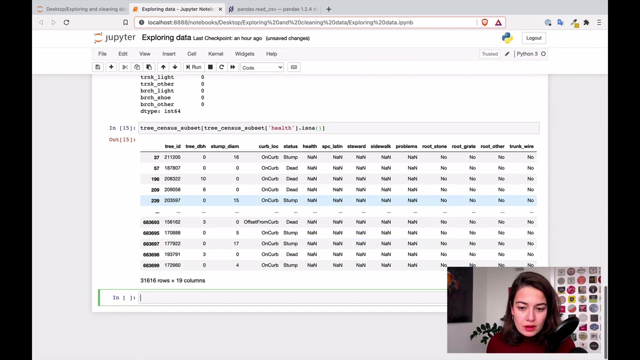 683 rows And out of the 683.. 31,000 is missing for these columns. So I want to see what it looks like when these values are missing. So I'm going to say: show me all the ones where health is a none value. 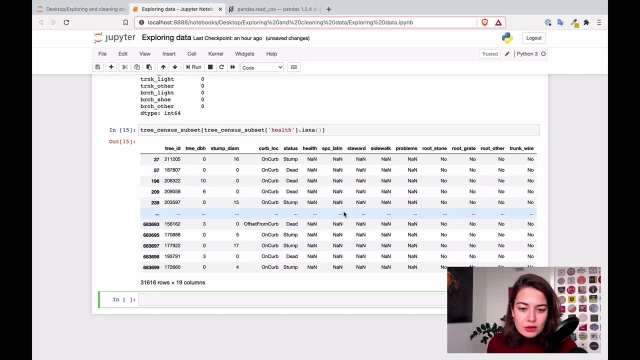 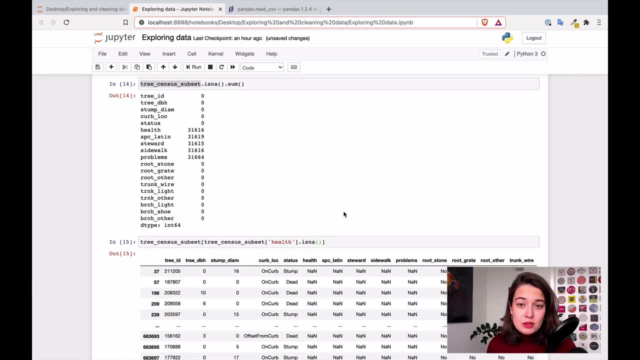 All right. So it looks like they're kind of like none for the same things. I can decide to remove these values later or not. That's kind of up to me at this point. But you know, I'm just exploring, I'm not doing, I'm not taking any action. 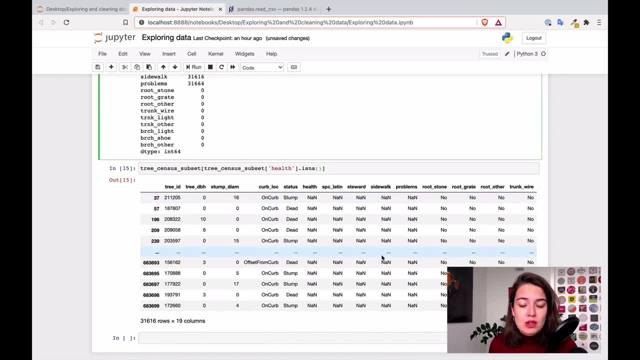 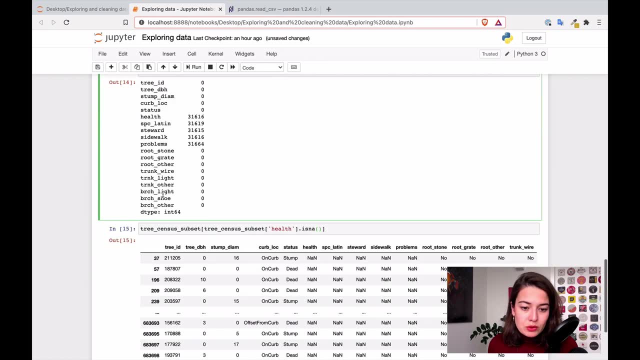 So this is something that you can take note of. You can say, hey, there are a lot of missing values, I just want to get rid of these ones. Okay, this is good. So let's do describe to get the general feel of the data set. 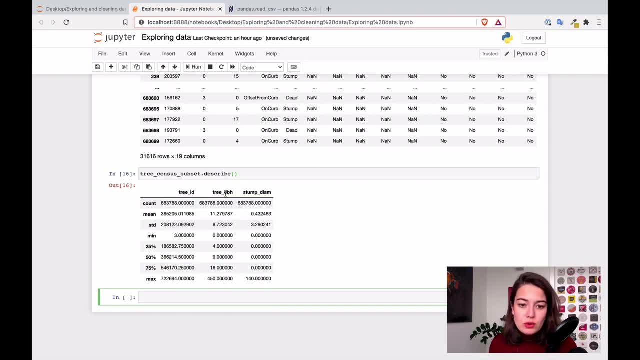 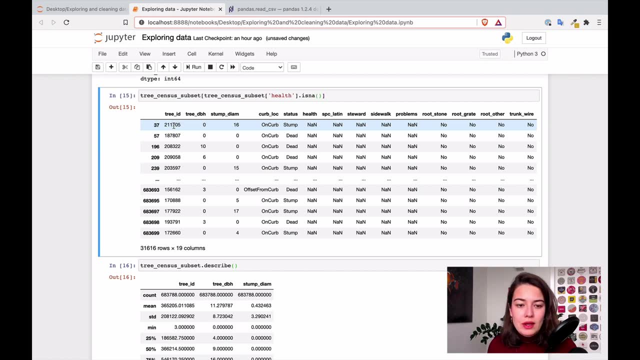 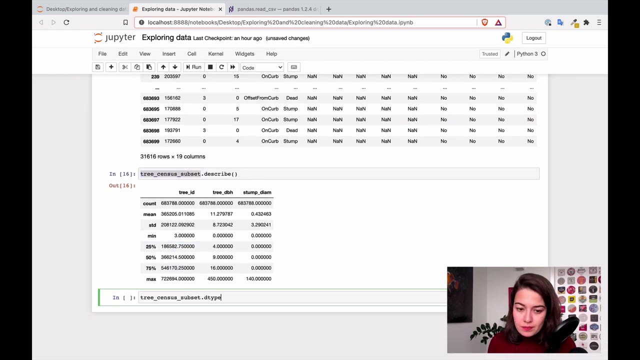 Okay, so, as I said, we only have two numerical values. Well, the first one, tree ID, is actually a categorical value Because it's the ID is not a continuous value, But it's currently sees it as numerical value, And we can see that if we do D types here, most of them are strings. 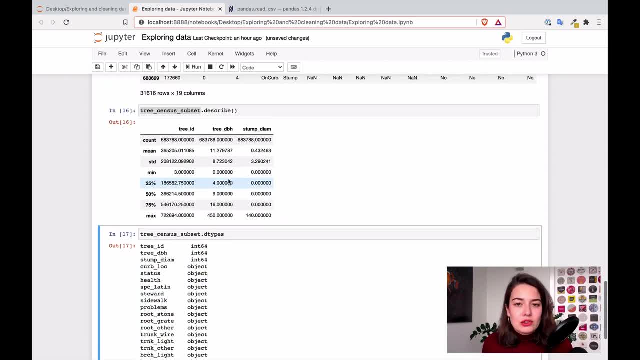 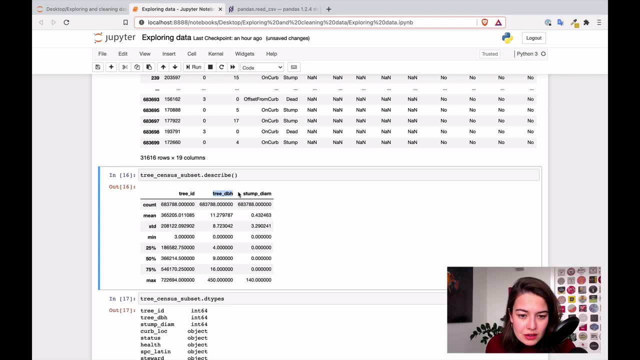 But the first one is an integer. So it's an integer because the ID of the tree- but it's actually should be a categorical value. So what I'm looking at is here the tree diameter and stamp diameter. So yeah, we have these many values. 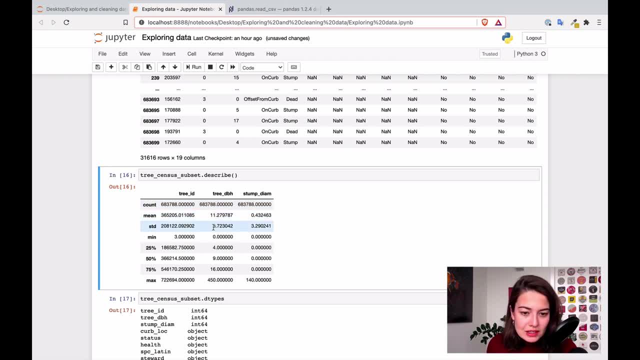 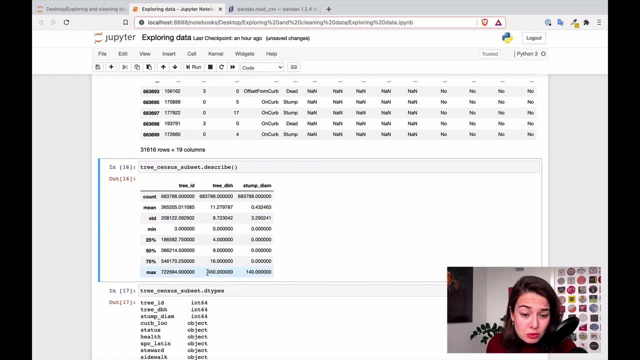 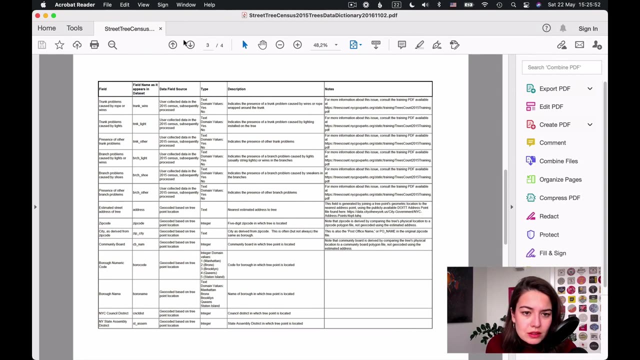 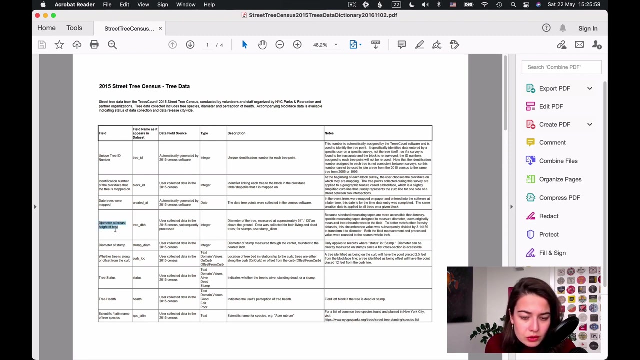 The mean is 11 centimeters. standard deviation is eight centimeters. Okay, These are some tiny trees And maximum is 450.. That's really interesting, Is it? centimeters? User collected the diameter of the height of the tree: integer diameter tree measured. 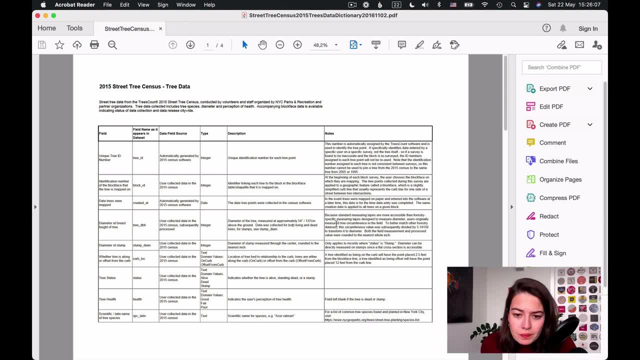 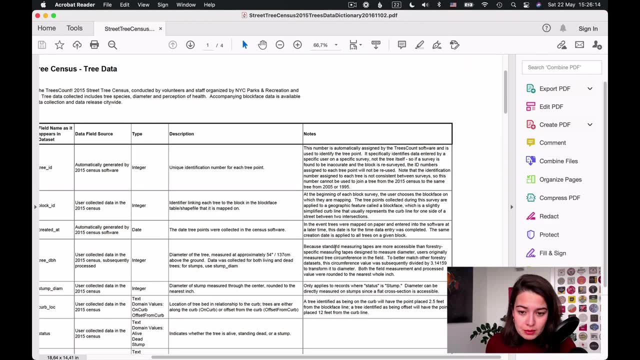 That's called the blood living trees. Um tapes are more accessible than forestry specific. Let me make it close Because I'm measuring tapes are more accessible than forestry specific. measuring tapes designed to measure diameter. users originally measured tree circumference in the field to better. 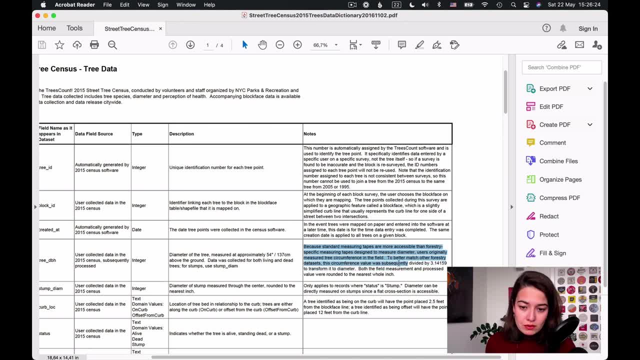 match other forestry data sets. The circumference value was subsequently divided by the pie to transform it to diameter. Both the field measure meant and process value were rounded to the nearest whole inch. So okay, It's not a centimeter, It's an inch. So this is important knowledge for us. I don't know what an inch is, So one inch in centimeters is 2.54.. So that actually is like even more in centimeters. So if it's like a hunt, 450 inches, that's like a lot of centimeters, 450 inches in. 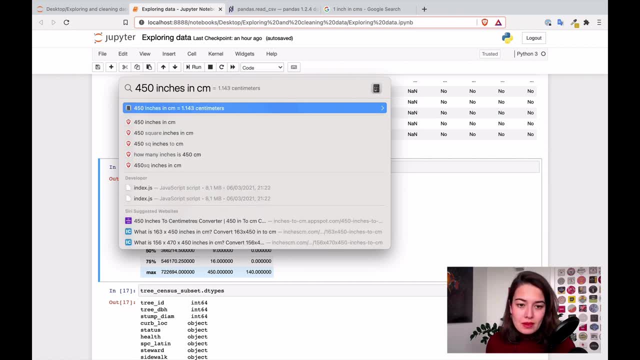 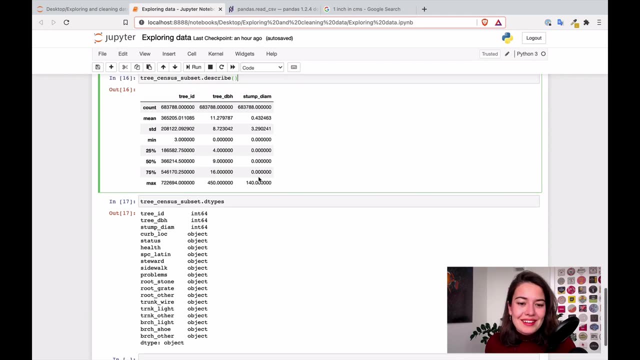 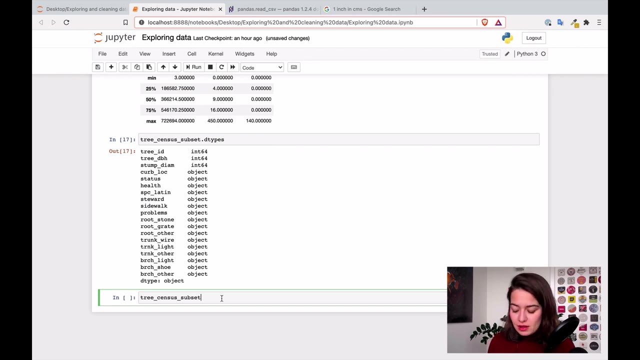 centimeters, even, Um, okay, Okay, 1000 centimeters. It doesn't sound likely, but let's take a closer look at this actually. So what I'm going to do is I'm going to create some histograms, because I want to see the distribution. 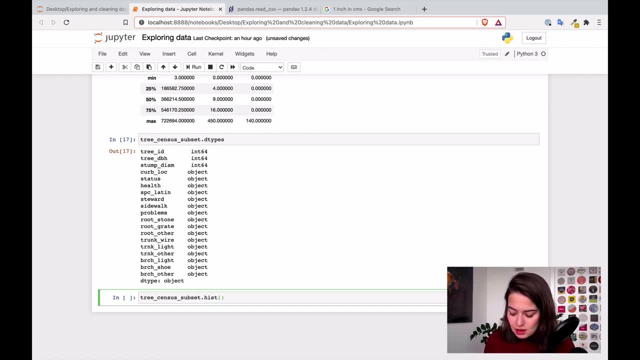 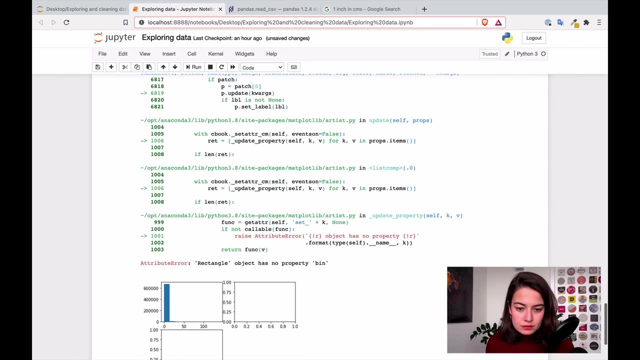 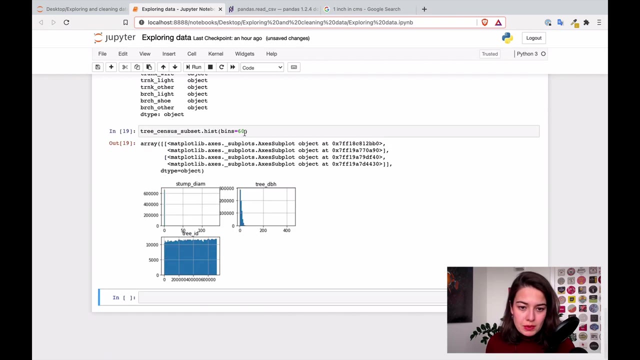 of these values. So let's say hist, And I already want to make the bins a little bit bigger- Hmm, Okay, Yeah, it's bins- And also want to make the figure size a little bit bigger. All right, It's interesting. 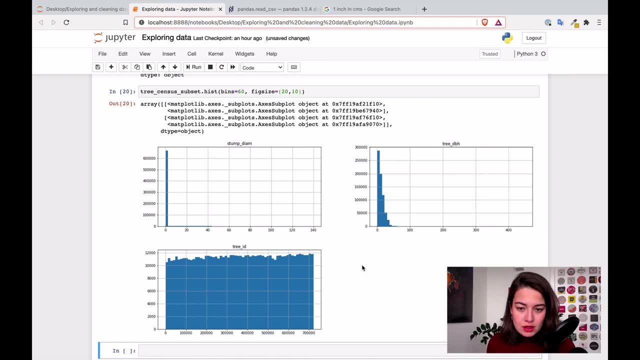 So, again, I'm not really looking at a tree ID. As I said, it's not really something that's uh important. Stump diameter: uh, it's close to zero most of the time, but then uh, I don't know if. 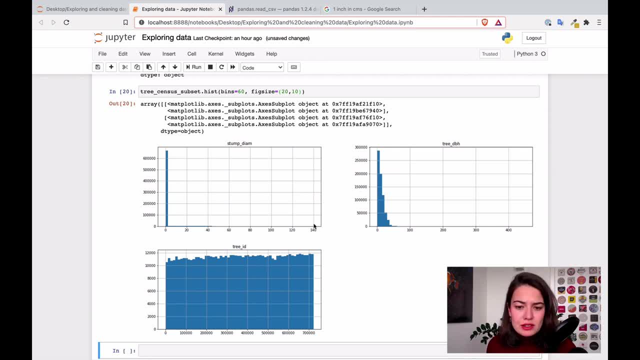 you watch some other videos of mine, But I think I mentioned this earlier in the hands-on data science course. if you can see this value here, that actually means that there needs to be a value here, because that's how the histograms are being made. so if the maximum value 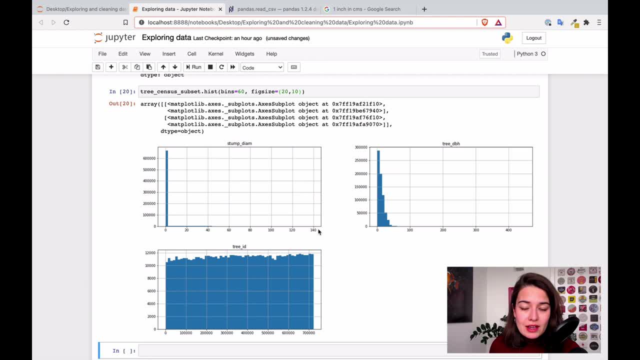 was 60, the histogram range, the x-axis range, would be from 0 to 60, but if if it goes to all the way to 140, it means there is a value somewhere here, even if it's just one. uh, same thing with the three diameter. so i think something went wrong there, probably when someone was trying to 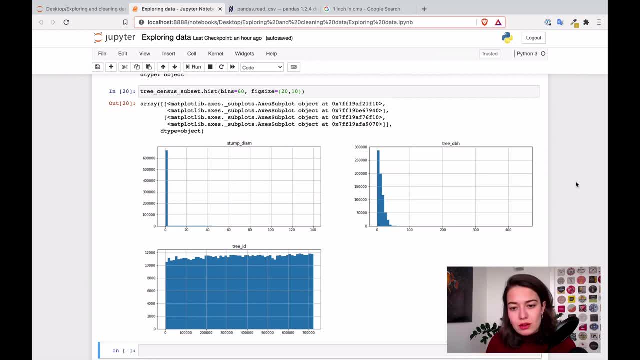 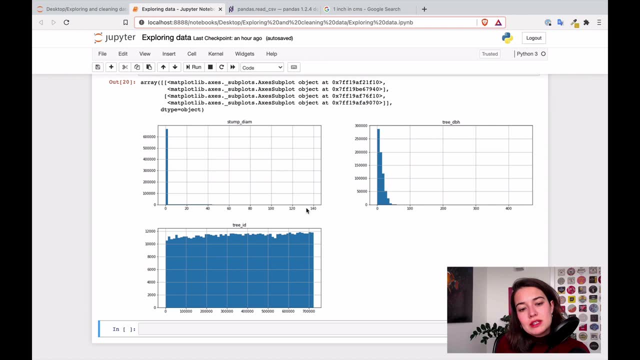 you know, put the value in. they actually want to write like 45, but i accidentally wrote like 450, so we don't know that. so i also want to see, like, how many values are here. or how many values are here- so it looks like a logical way to cut this off- is maybe like 40 here, because, as you can see, 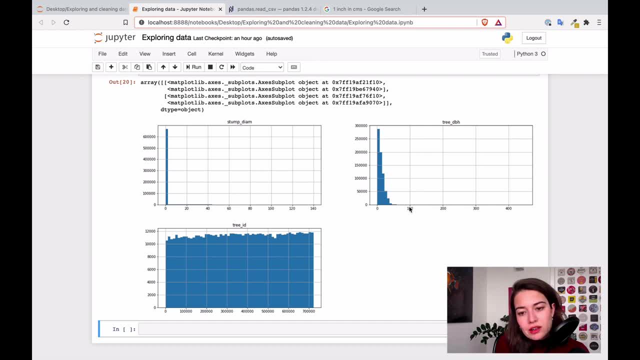 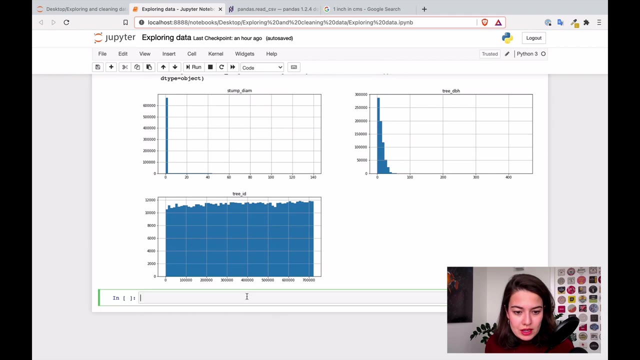 there are still some values here and also maybe like 100 you inches here. even that sounds like unreasonable to me, to be honest. but um, so let's see, let me. let me visualize that a little bit. so what i'm going to say is: give me all the trees where the tree diameter. 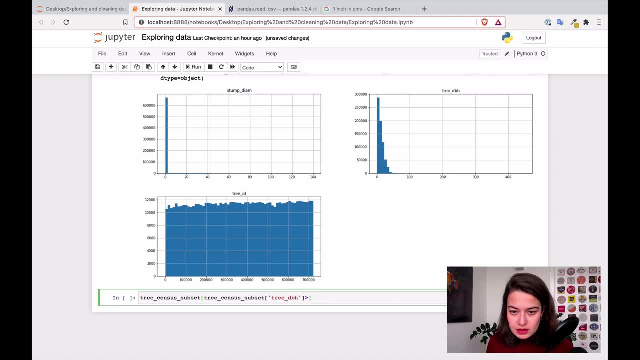 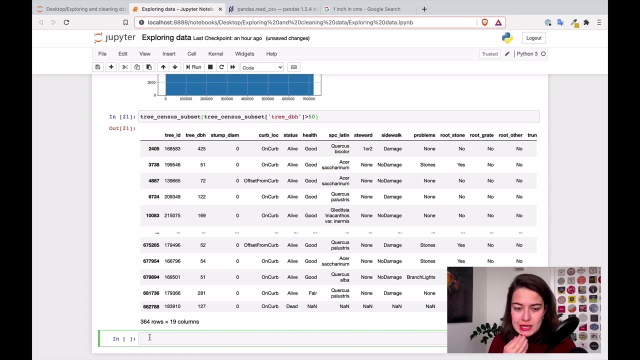 is bigger than we're going to say- like 50, to be honest. so we have 300 pop, perfect, not 300 or more. it's going to be. it's going to be day. uh, that looks like a tesla. that's a really nice day add-on. so i'm going to kind of top it off there and i'm going 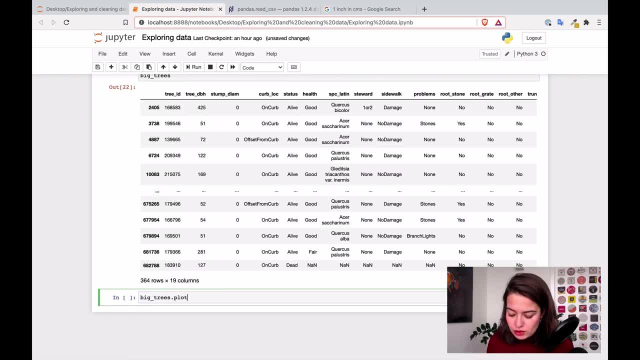 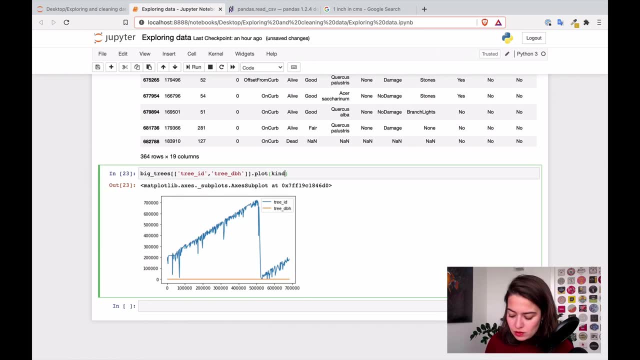 to just say, the value on the bottom right hand side of the graph is the gradient value minus the main value. so this will become the median of the bar per square. this will become the volume of d given by the protocols that we have, which is apply. so here, if i convert this layer to a 500, 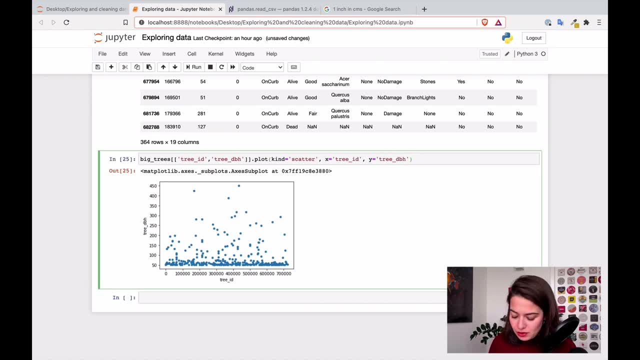 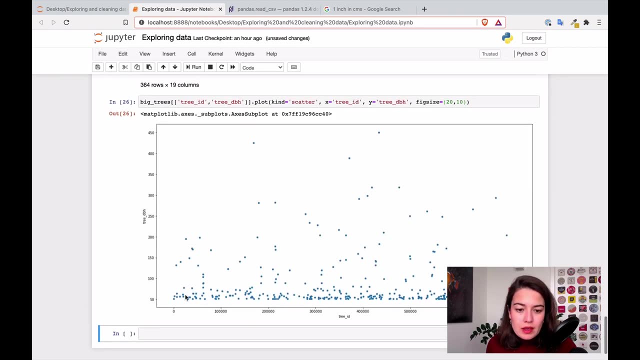 okay, this is more or less what i expected, but let me make this figure a little bit bigger. yeah, there are some here which i guess is expected, but, like especially after here, it's kind of like you know they're one or two trees. this, uh, seems very silly to me that there will be a tree. 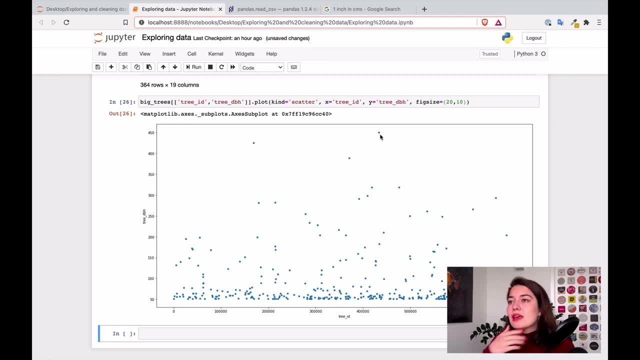 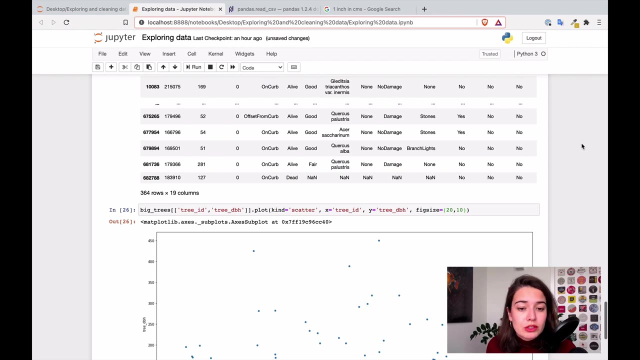 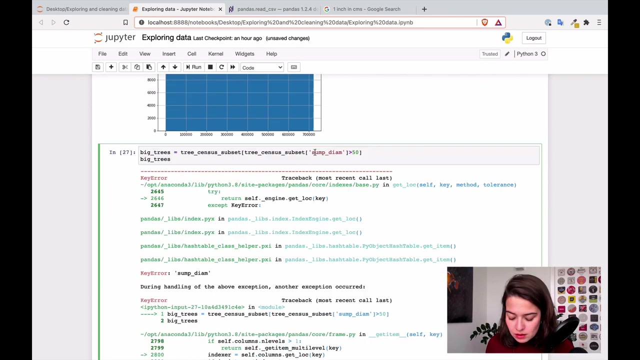 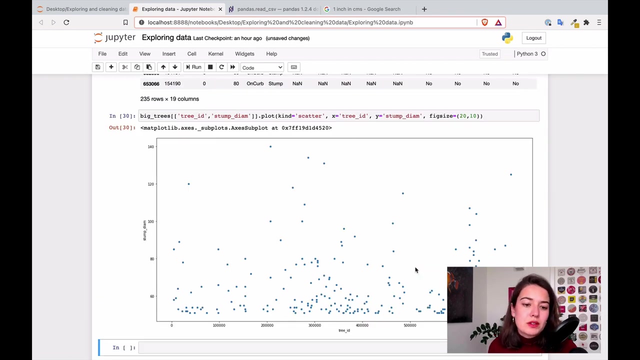 whose diameter is 450.. i mean, yeah, even even the circum circumference, 250 inches, sounds like ridiculous, uh. but yeah, this is just some information that we have right now. good to know. good to know, um, we can do the same thing with the stump diameter. all right, similar, similar thing. i guess, maybe, until up until this point, it's acceptable. 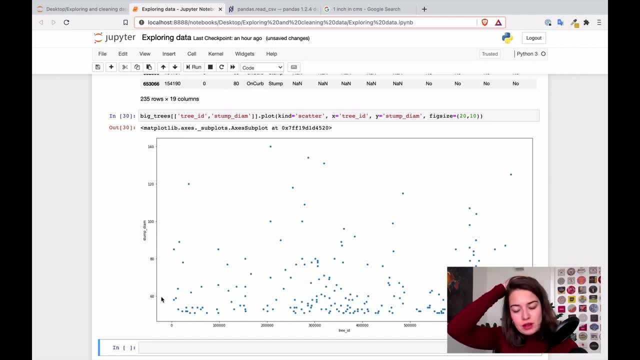 maybe they forgot to change it to diameter. they put in the circumference and yeah, and these values are kind of like not really correct- could be, uh, yeah, all right, i mean, i guess 140 inches is not unreasonable if it's uh the circumference and they forgot to put it into diameter. otherwise it should be like a very 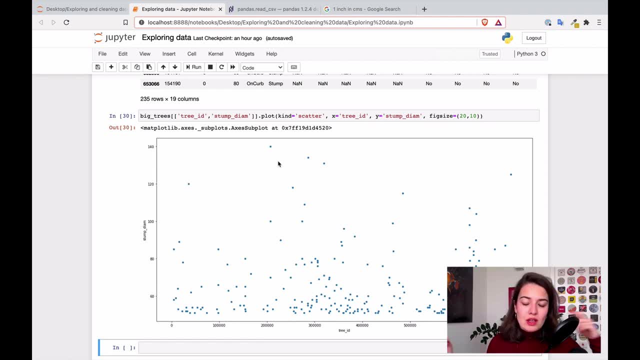 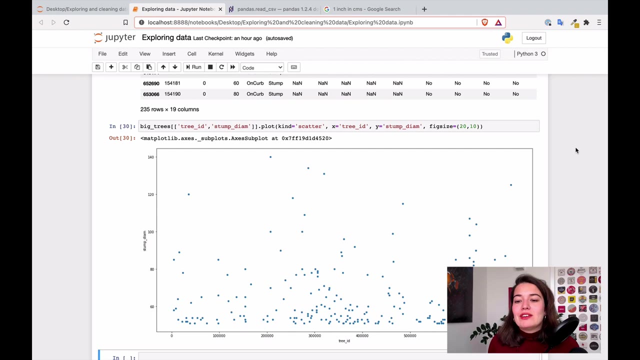 big tree, right, if the diameter is 140 inches and that makes like a lot of centimeters, that makes like three meters or something. a three, three meter diameter is kind of like yeah, that would be a bit too big. i guess i'm just trying to like work it in my head, you know, i'm trying to understand if 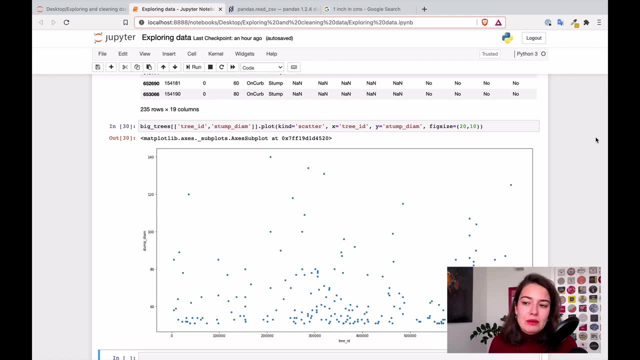 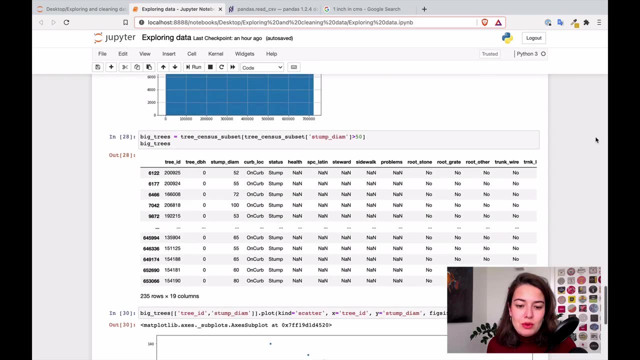 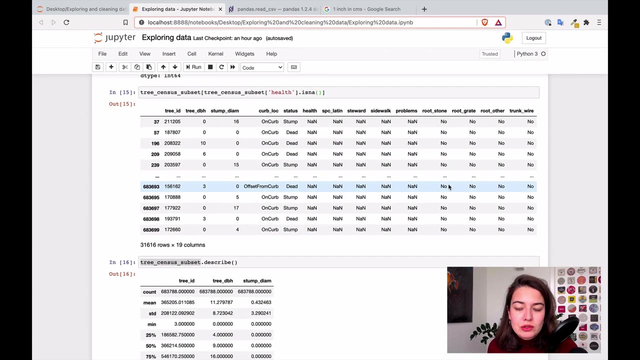 that's actually unreasonable or not. but yeah, when we move to the cleaning bit, i guess one thing that we would need to ask ourselves is: is this really unreasonable, is this not really unreasonable, and what can we do with this data point, or data points um? what else do we want to look at? i want to see what are the possible. 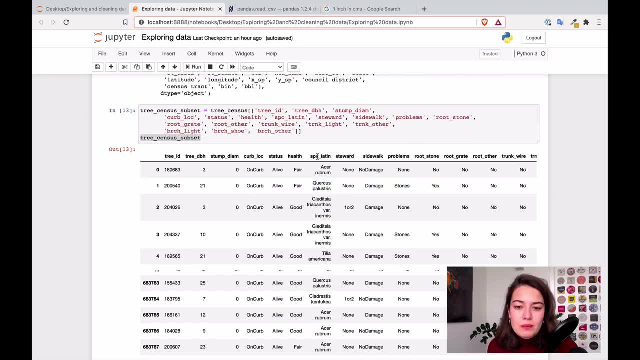 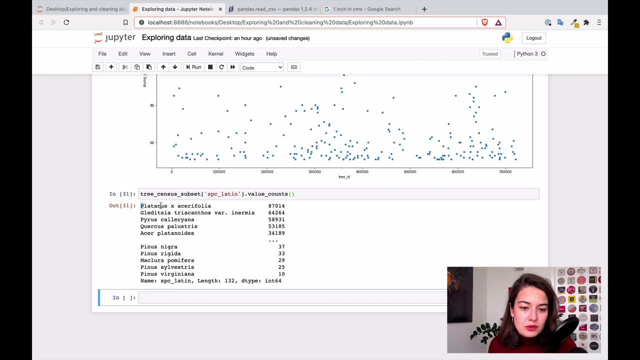 options for some of these other columns. so latin name: probably there are a lot of different latin names, but you know it could be interesting to see the distribution of different names. so i'm going to come here and say, okay, i guess this tree is very common and then we have less common trees here and one thing you can do to visualize this: 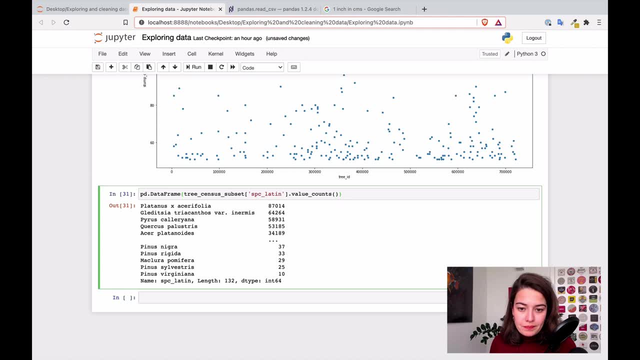 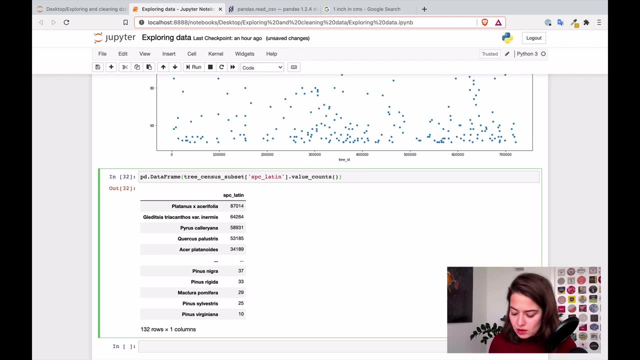 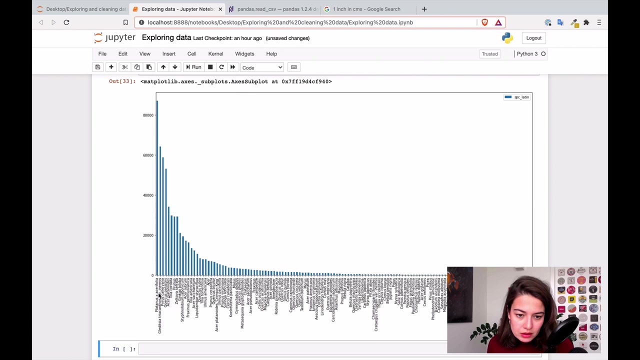 is to turn this counts into a data frame and then plot it. or maybe not histogram, uh, i guess plot. let me try a bar chart. that should work, i guess. yeah, okay, cool, yeah, i mean not the most readable chart in the world, but at least it gives you. 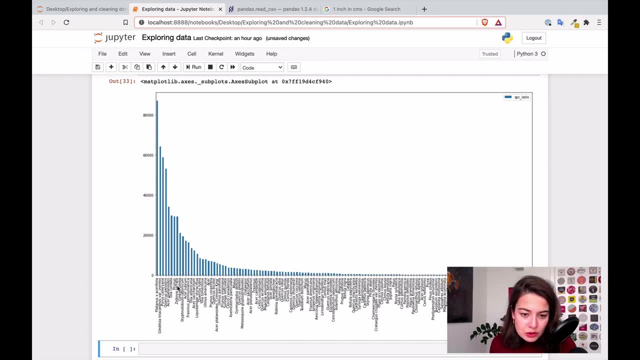 an understanding of you know how many trees there are and which types there are, and this is kind of expected, right? you would expect some trees to be like very common and then, as you go, it's like less and less common. all right, what else can we look at, so um? 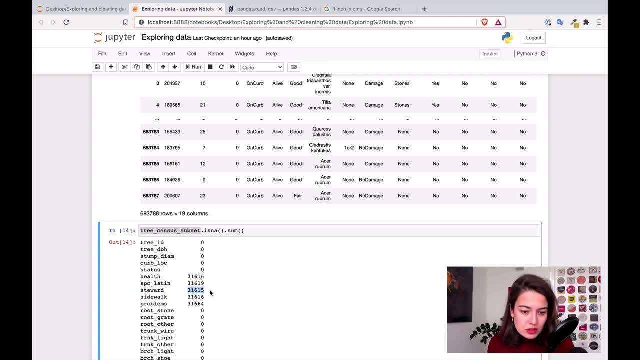 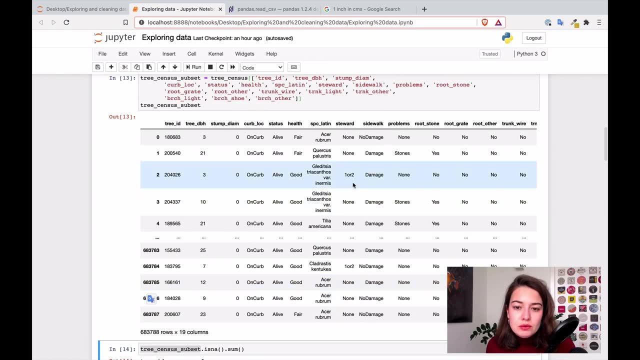 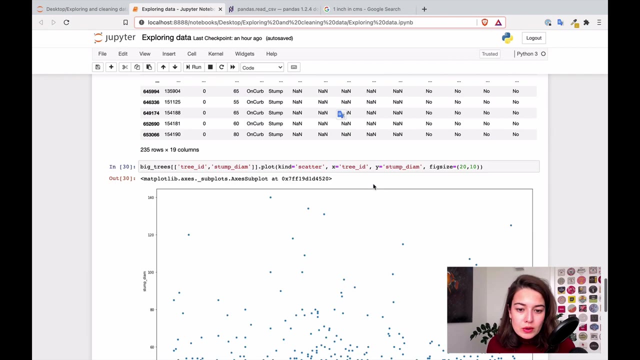 i saw that, yeah, there are stewards, right, some of the values for the stewards are missing. uh, sidewalk is missing, a problem is missing. but I want to see, like, what are the options for stewards? so we can see here one or two or none, but what are? what are some options? 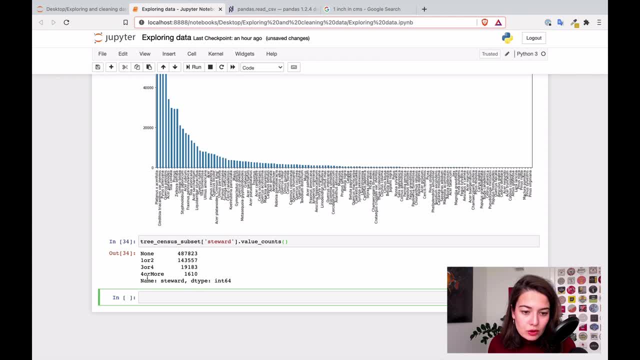 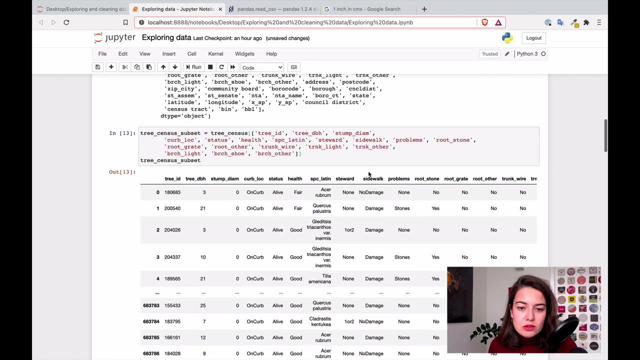 okay, so it's either none, one or two, three or four, four or more. this is good. it looks very standardized. so you know, if everyone had to write it down by themselves, you can see someone writing one or two, someone else writing like this, someone else writing like this. so it's, it's possible. it's good to see that. 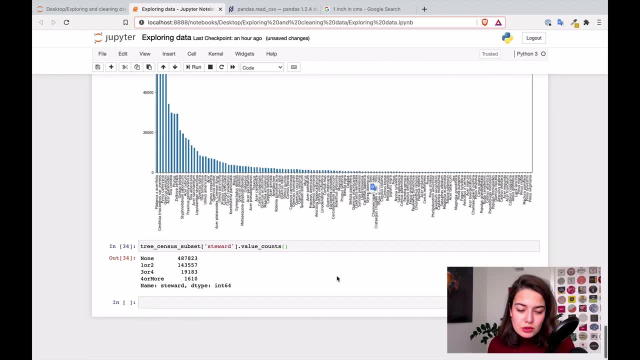 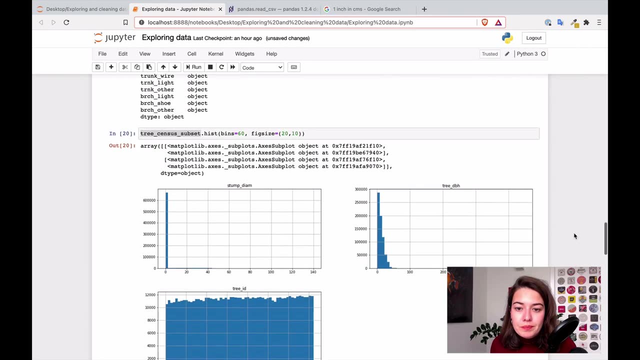 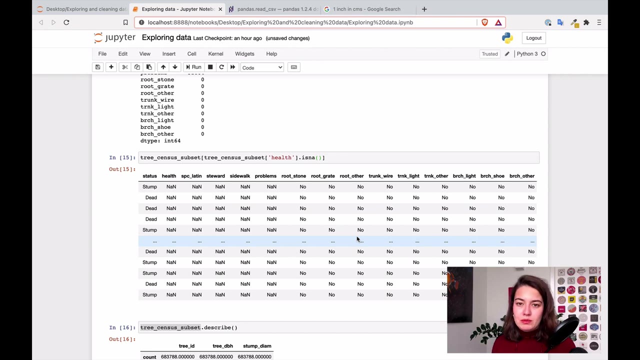 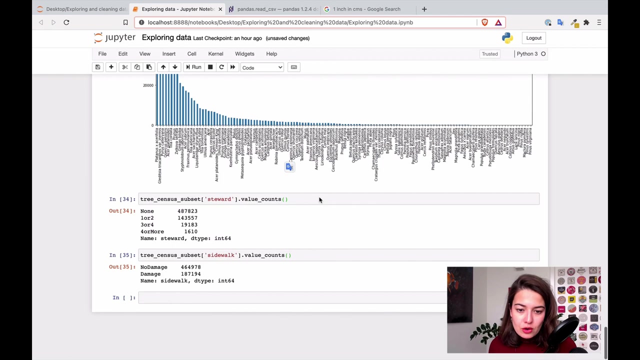 it's clean. I want to see the possibilities for sidewalk and no damage or damage. okay, good, mm-hmm. I guess for these ones is either yes or no. I'm guessing this could be like a you know website where they feel in a form, so this looks pretty standard. I want to see the status and curb. 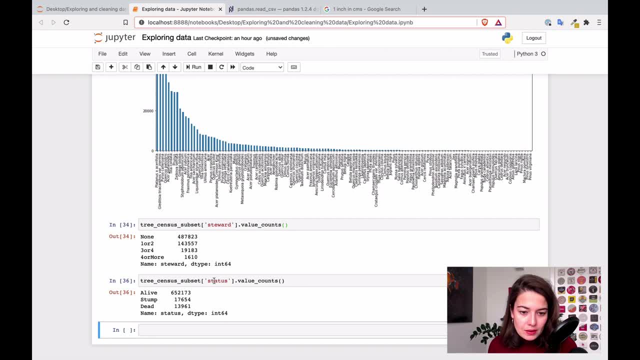 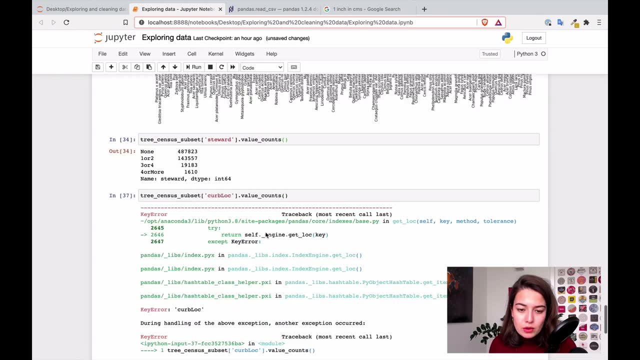 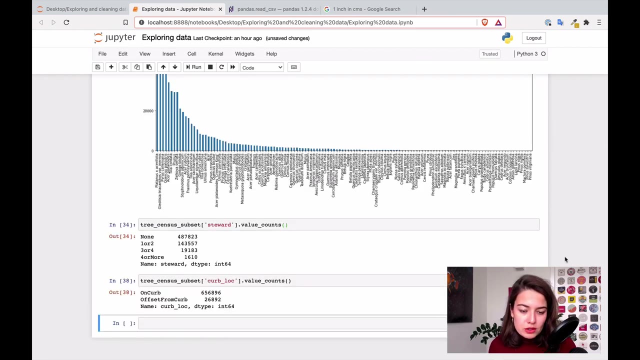 length and I want to see the status and curb length and curb length and curb length location. also, let's do it quickly, uh-huh. curb lock, was it? no, what was it? curb lock with the underscore on curb or offset from the curb? okay, cool, doesn't? 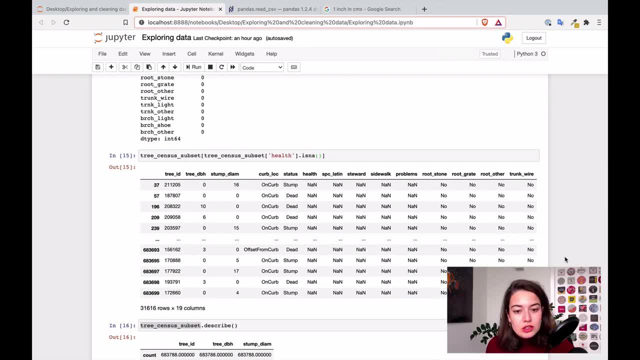 seem to be neat for extra correction there, all right. one last thing that I want to look into is if there is some mismatch between, you know, this tree being a stump and the health of the tree, for example, if there is any point where it says it's a stump. 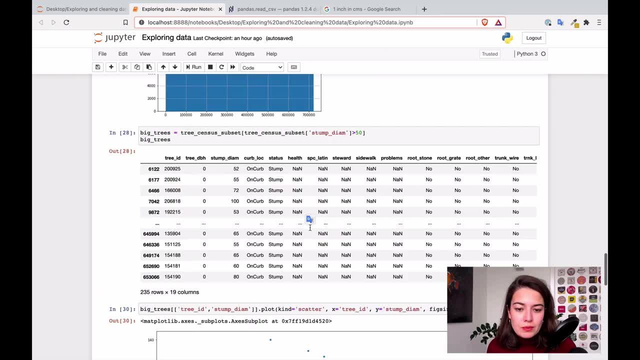 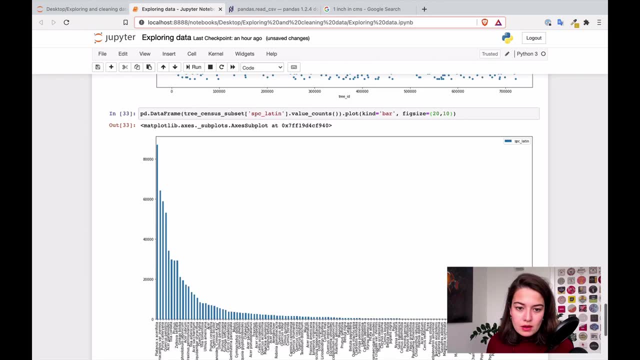 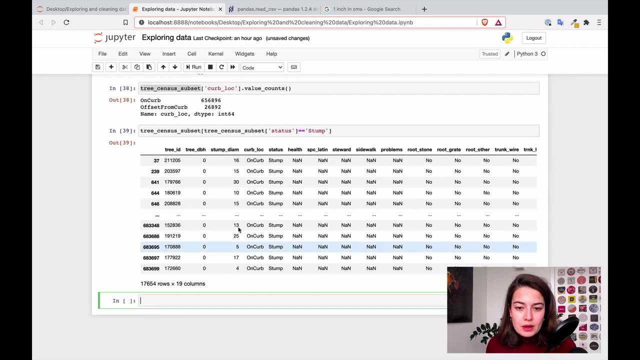 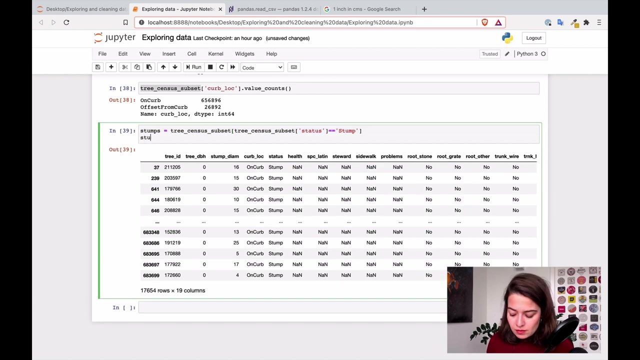 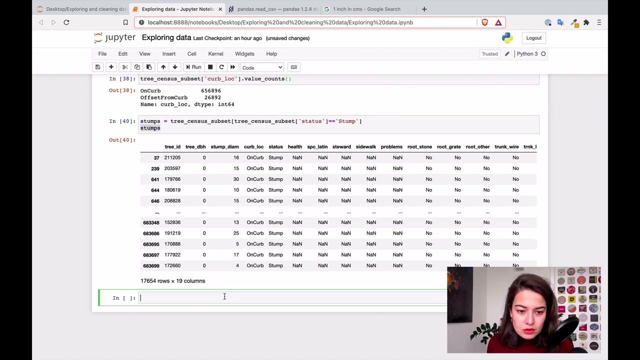 but it says like health is good or something like that. so I want to get all the trees where what is the name of that column? status is stump. okay, then you know, then I can say stumps. so this is like a new subset and all the value is none for the stumps. no, oh so maybe these like stewards sidewalk. problems, health stuff, are none for all the stumps and all the dead trees. so let me check that. for the dead trees that's Hmm. so how much does that make? So you know, there are 17,654 stumps, it says, and 13,961 dead trees. 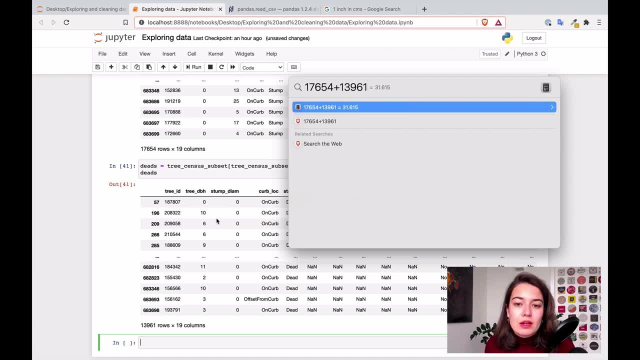 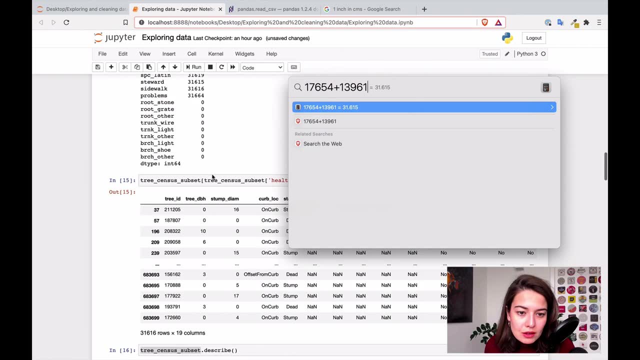 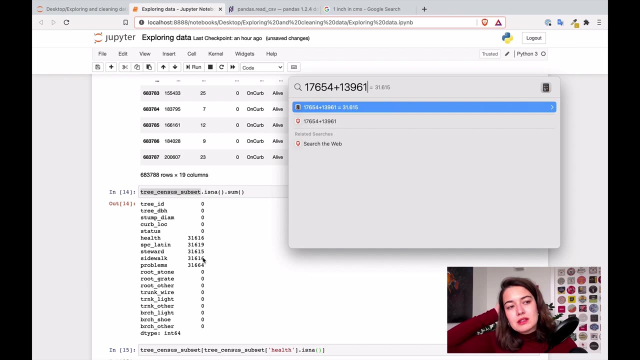 That amounts to 31,615 total dead or stumped trees. So, basically, how many values did we miss? Yeah, it's more or less the same. So I guess what happened is, if the tree is not alive, they didn't either bother or they. 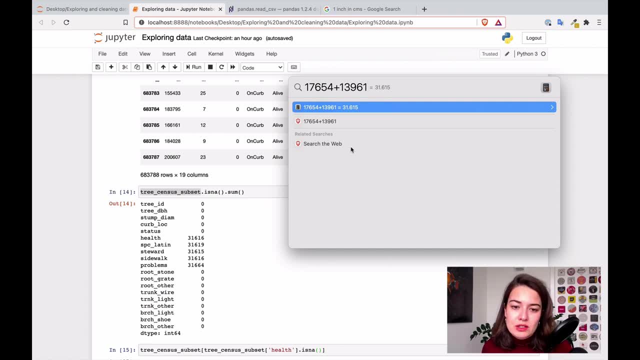 didn't think it was relevant to fill in the information. for the rest, for the health Latin name: steward, sidewalk problems, etc. And probably for these ones it just like put zero or something like that. Okay, so that's good to know. 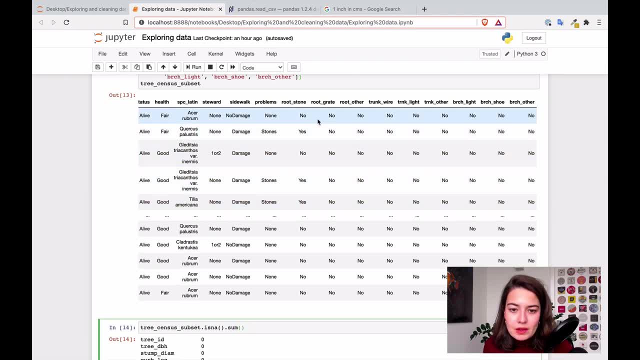 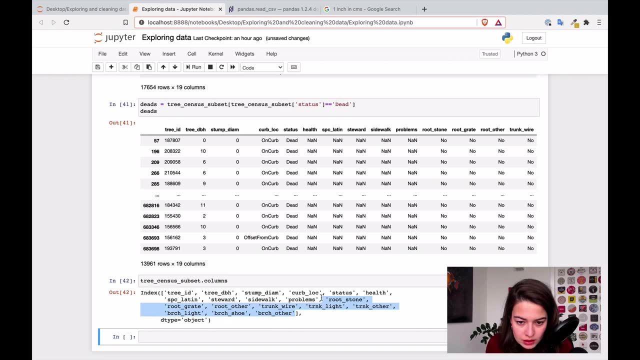 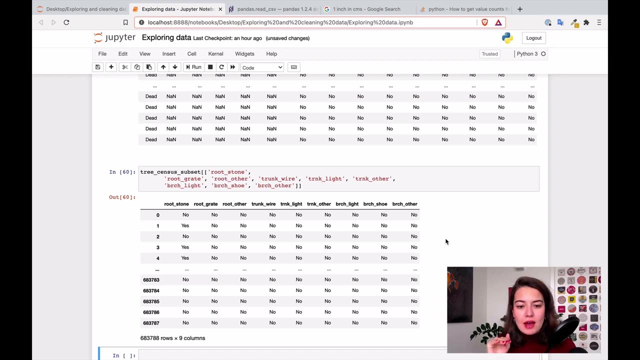 And also one other thing that I want to look at is how these guys are distributed. Okay, so what I want to see is actually how many yeses and how many no's there are for each of these columns. Of course, it's going to seem really instant to you that I achieved this, but I actually 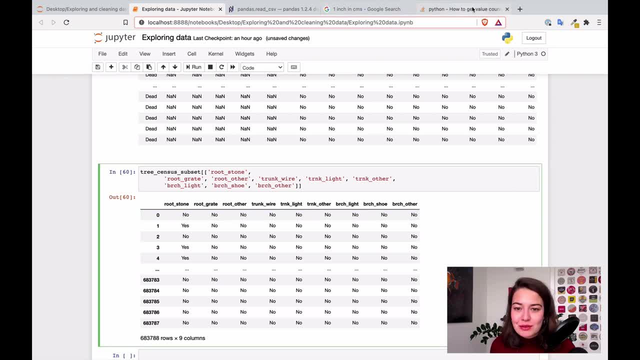 took like 20 minutes or something looking online to see- as you can see from my searches here- how I can see this information. So basically, I found that out. So what I need to do is just assign this to a data set. 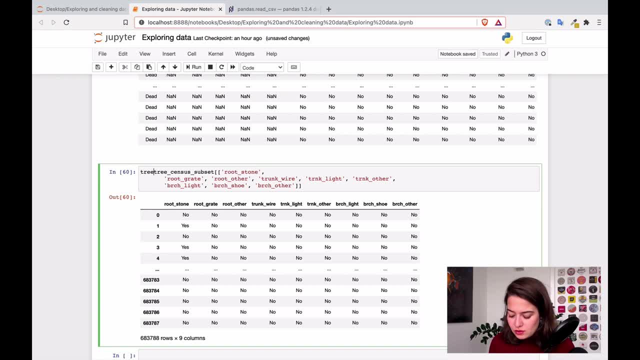 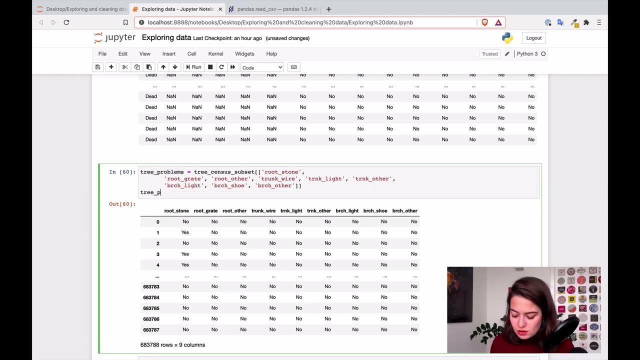 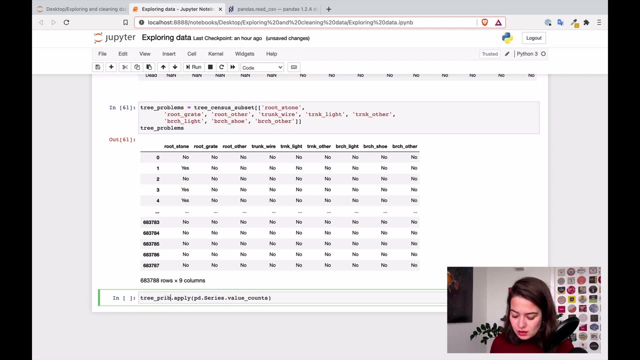 What should we call it? Tree problems? let's say So. this is a data set, And apparently the way to see it is like this: Just apply the value counts function to each of the series, And then you're able to see the values for all of them. 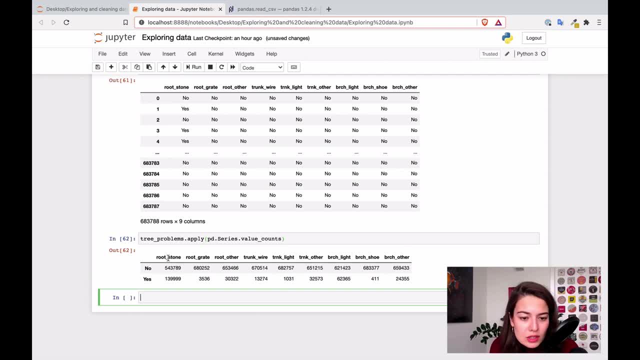 So okay. so let's see, It looks like root stone problems seem to exist a lot of the time. Yeah, no other problem exists that much. So yeah, So problems caused on the root by stones is a big problem. Yeah, this is just good information to have. 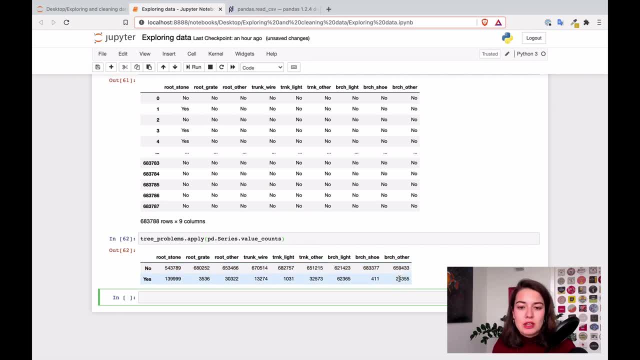 You know, these are also things like when you're starting a project. These are some information, some statistics, that you can give to whoever is responsible for the project, or if you just want to kind of show that you are progressing with the problem or with the project. 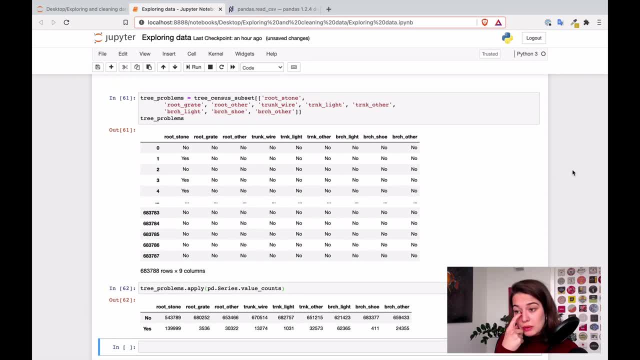 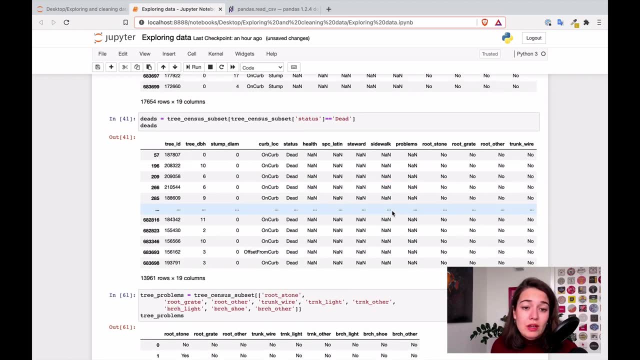 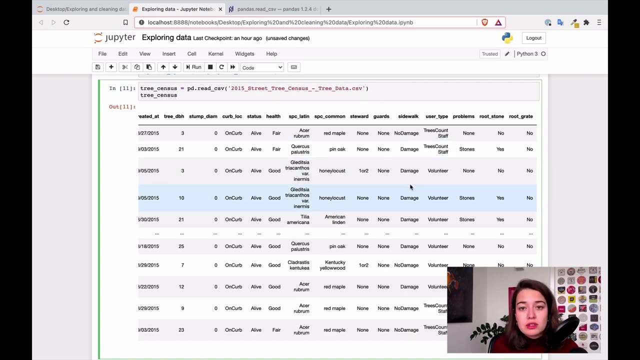 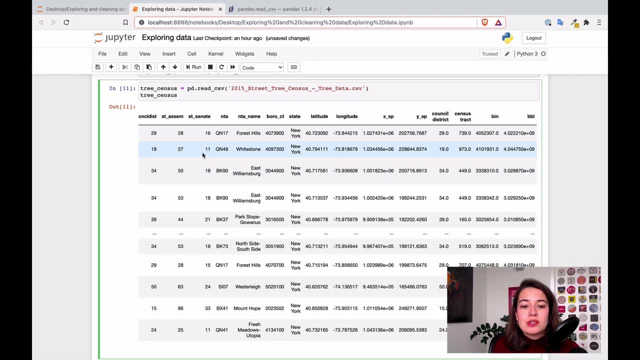 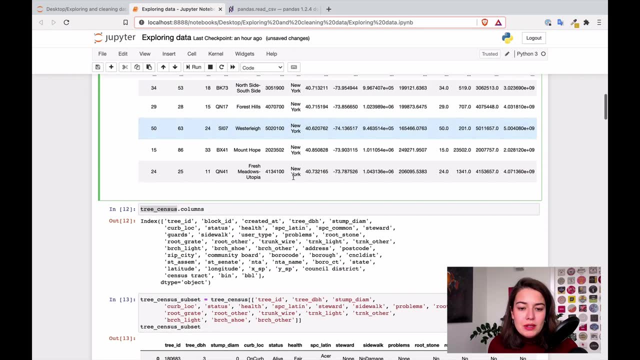 We decided that we don't really want to get into the details of where the tree is located, which borough is responsible from the tree, which street it's on. So we haven't been looked, we didn't look at it, didn't look into that because we decided that's not important for our purposes. We 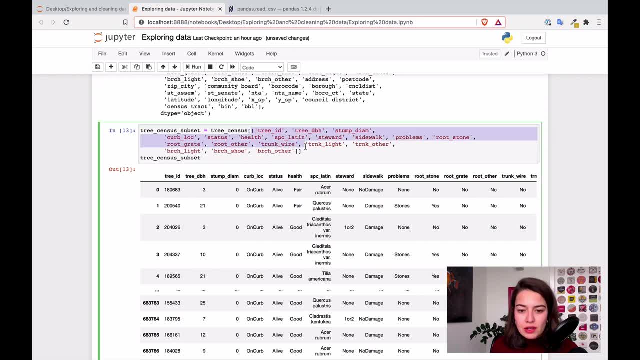 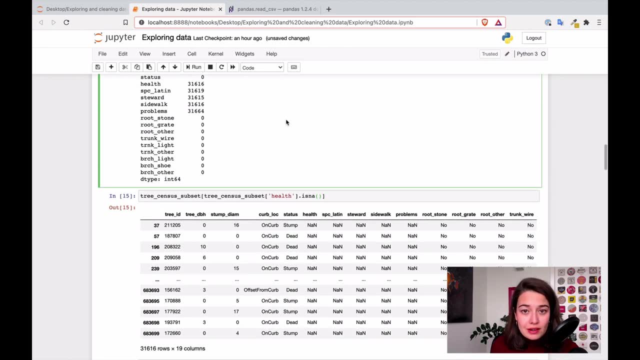 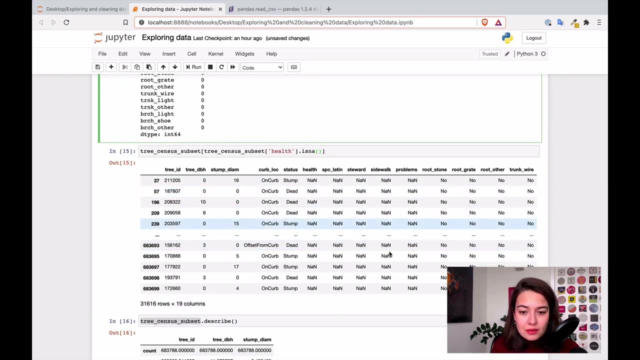 looked into the columns that this data set has. we chose the relevant columns only and on this relevant columns, we first looked into the missing values. Again, we haven't done anything with these things yet. that will be in the next video- And we looked into, you know, if these missing values happen all at 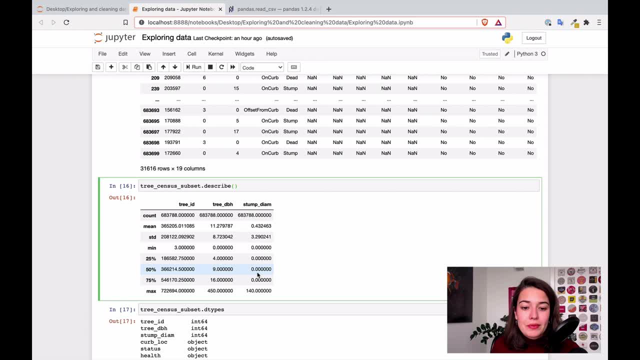 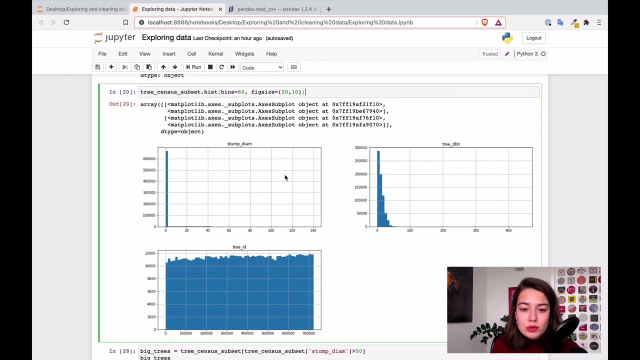 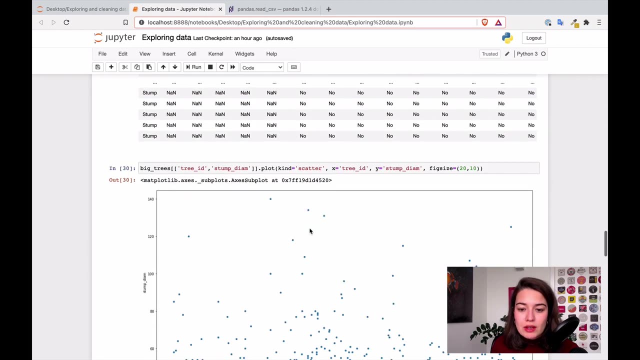 the same time or not? Then we looked into the numeric values and how they're distributed in general. We looked into the distribution, the histogram, and saw that some of the values are looking a little bit suspicious. So we went deeper in those values and looked: how many of them are this outrageously high? 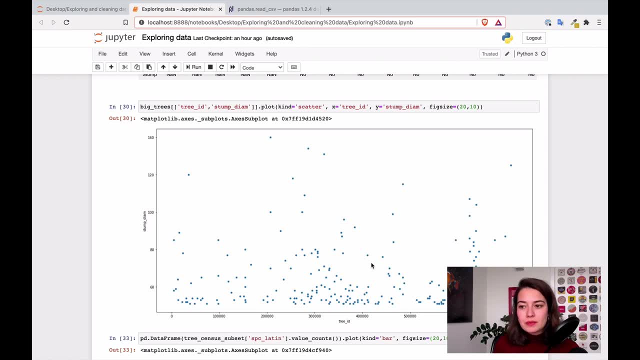 So if you saw a really even distribution here, that there are a lot of dots here and there, then you might think that our maybe this is normal to have. But when you see there are only a bunch here, kind of like outliers, then you can decide maybe this was a mistaken input by whoever was. 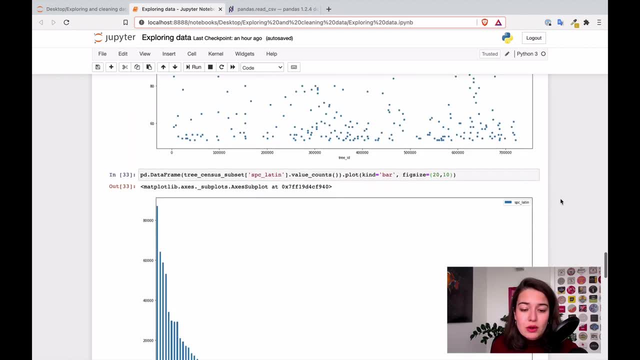 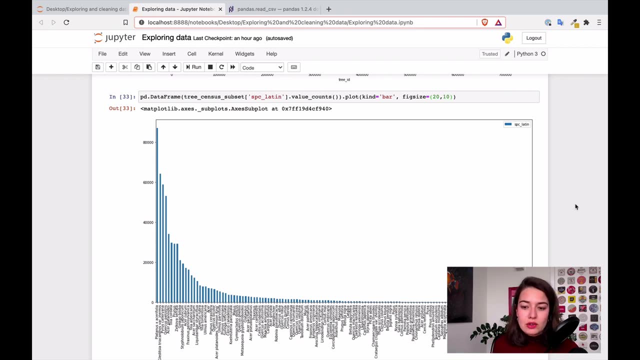 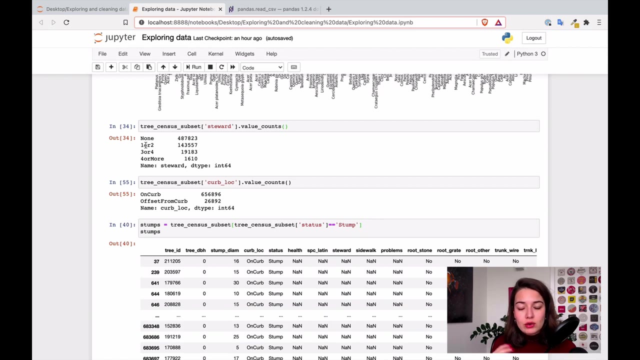 collecting data, Same with stumps that we saw there. Then we looked into some names, how the distribution of different types of trees is in New York City and some just to make sure that all the a categorical values are are standard and there is no different terminology. you know, as I said, from one to two there's not. 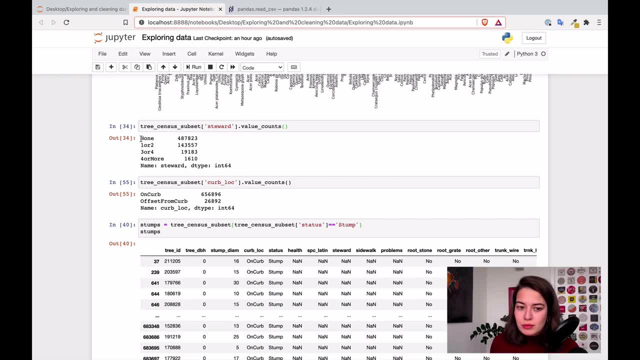 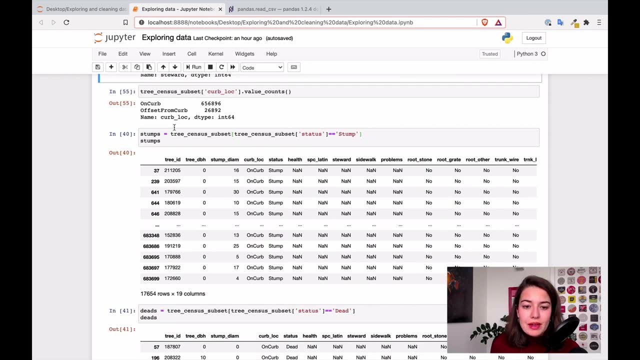 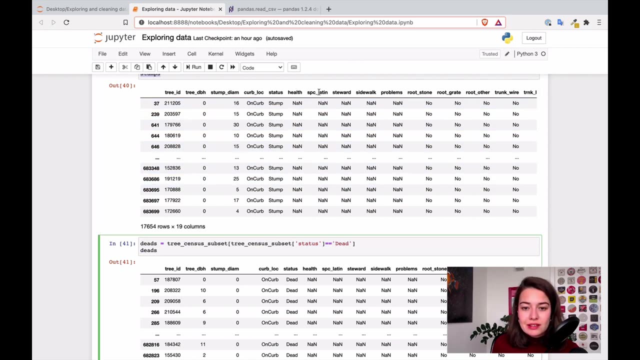 like one dash, two or anything like that. so just to make sure that the values are standardized here. we looked at some of the or most of the columns and we actually figured out that when it stumps or when it's a dead tree, the information on health let names the whether it has a steward. 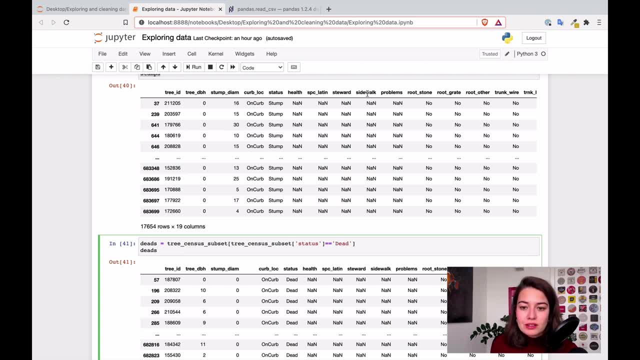 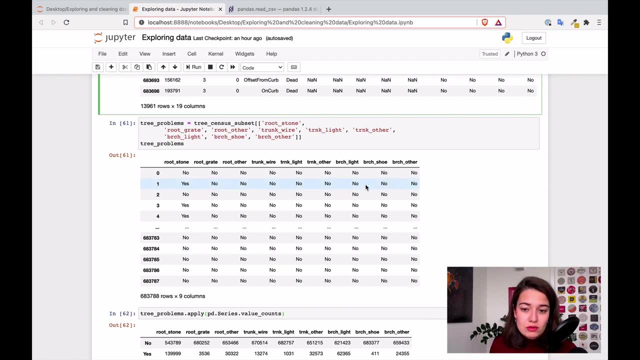 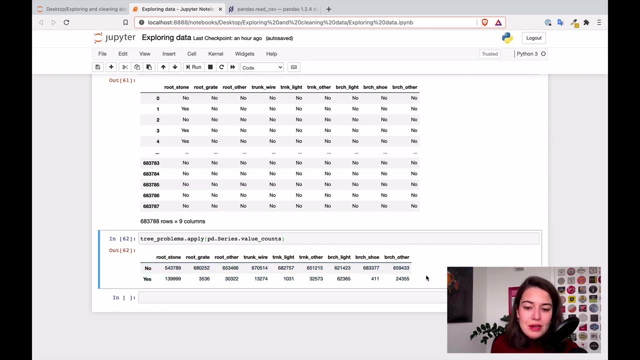 or not, whether it's on the sidewalk or not, etc. or if there are any problems with the tree. it has not been recorded. this is a good thing to know about the data set and we saw that the basic distribution or how many problems, what kind of problems there are on trees, so this is a good